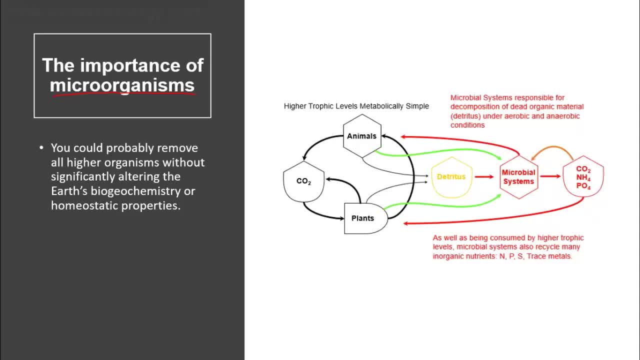 ecosystem works. Okay. so animals and plants, both are related to one another. particularly animals are dependent on plants because plants are the producers, So they're producing food and animal eats plants as a food source. Okay, and once animal X like animal, utilize oxygen. 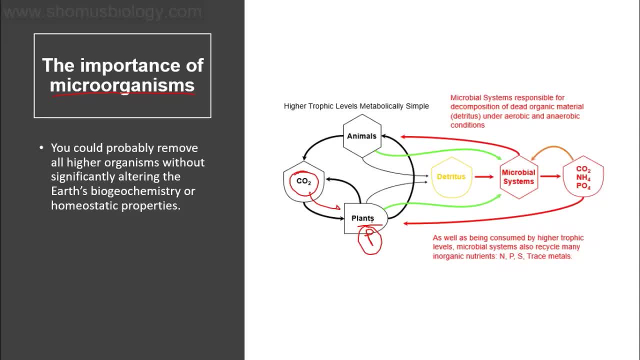 for respiration, produce CO2. plants take up that CO2, assimilate the carbon in CO2 into food And then, after the death of animal and plant- okay, they turn into detritus, and then. microbial systems means microorganisms, bacteria and fungi. both can act as a microbial system. 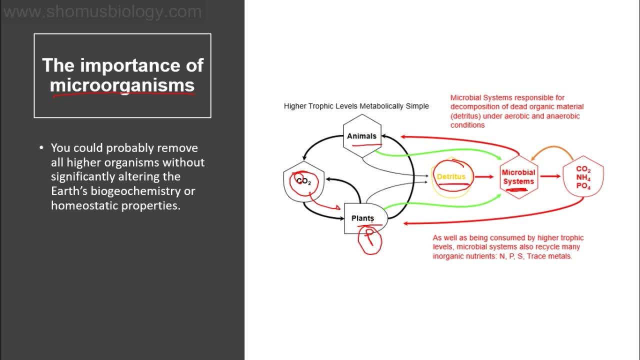 can convert the detritus into okay other components: carbon dioxide, ammonium, phosphate. these are the components that they produce, So microbial system responsible for the decomposition of the dead organic material, Which is known as detritus, under aerobic as well as anaerobic condition. and then they 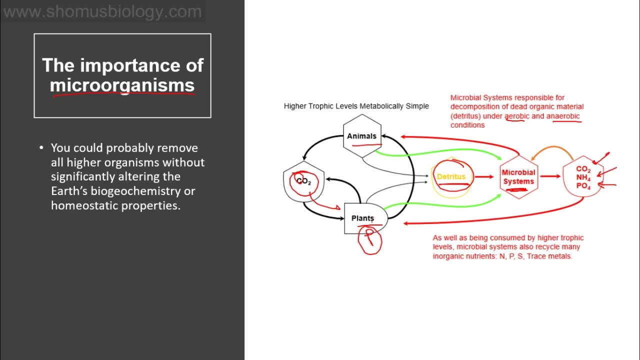 will produce components which will be again released into the nature, released into the environment, like CO2, NH4, PO4, those things. So, again, plants can take up this ammonium phosphate, because these things are present in the soil and CO2 is present in the air. 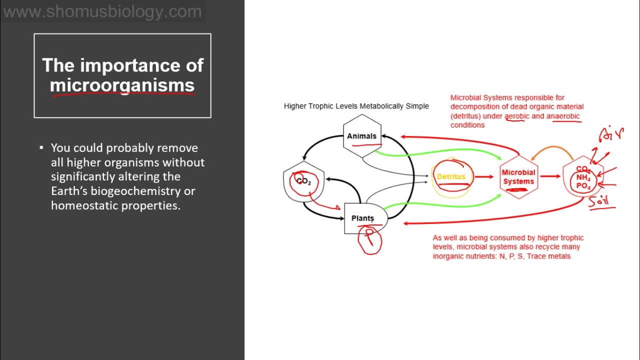 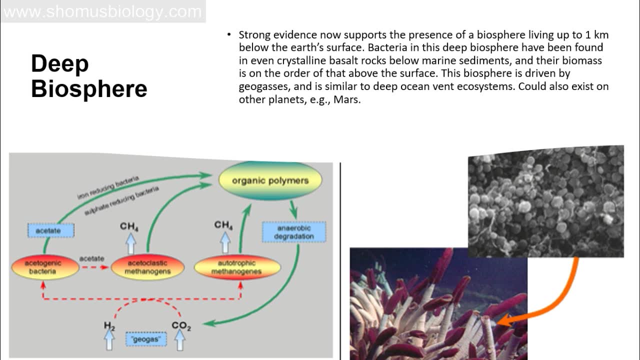 and plant in a, utilised it and produce food, and this cycle continues like that. So this is the actual functional role of a microorganism, Microbial system, in the environment. Now think about it. strong evidence now supports that. the presence of biosphere living up to one kilometre below Earth's surface and the 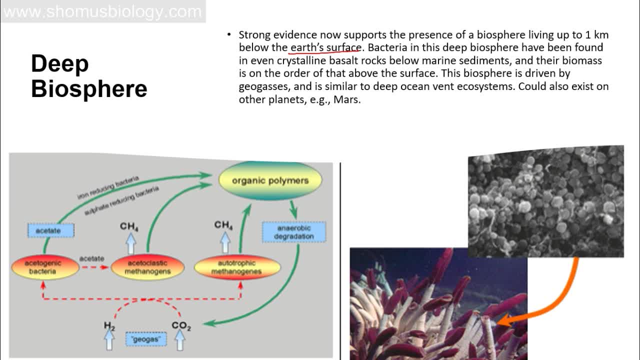 vector in this deep biosphere have been found in even crystalline basalt rocks below marine sediments, and their biomass is on order of the above of the surface. The biosphere is driven by geogases And similar to the deep ocean When. 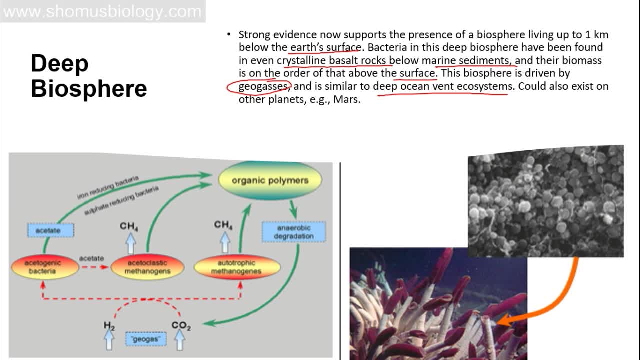 So think about it when we can find out microorganisms one kilometre below the surface, as well as you can find the one kilometre deep down the marine sediments. The similar type of environment is also present in other plants like Mars, and it is possible to find bacteria living. 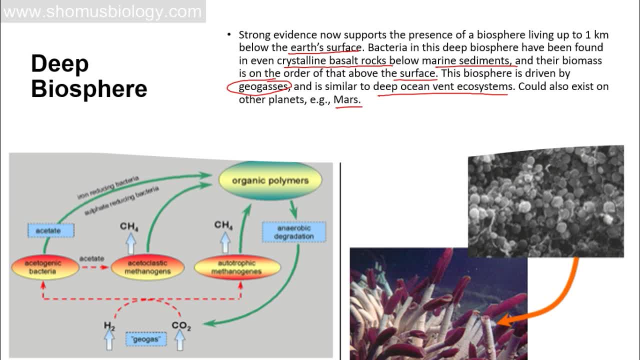 one to five kilometres down, the Mars and other planets surface as well. because these microorganisms They don't. They don't need solid food to leave, They need an energy source, They need a carbon source, Once they find that they can continue to leave, so that source of carbon they can obtain from. 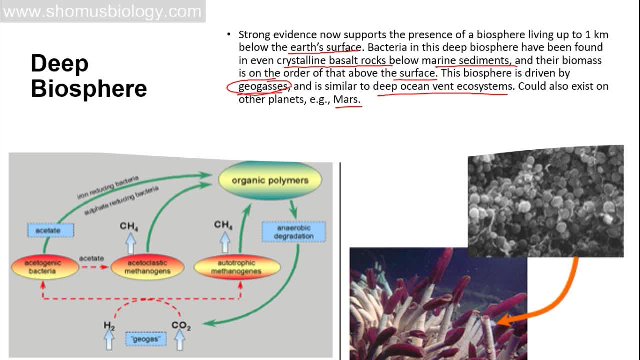 atmosphere from here. So geogases can provide them with this, nutrients with the carbon source. So think about it. You can have acetogenic bacteria as see to Classic methanogens And Autotrophic methanogens. okay, all this autotrophic methanogens and uh, aceto plastic methanogens. 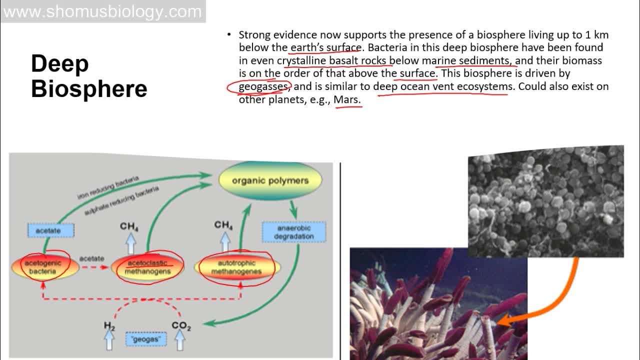 both these types. They are methanogens, means ultimately, when they utilize geogases like carbon dioxide or hydrogen gas, they utilize this gas and the produce methan and the remove the methan out and is methan, which is an organic polymer that can be again degraded an aerobically. 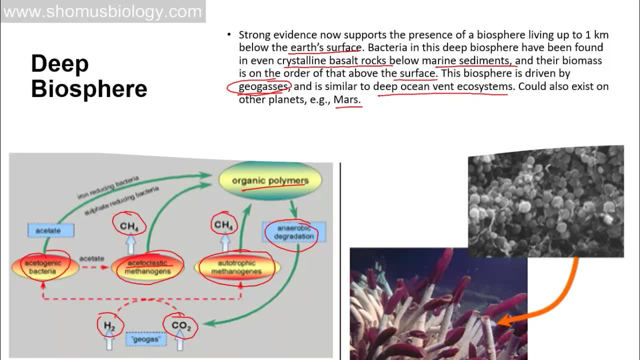 and further produce again carbon dioxide, Hydrogen. So it's a positive feedback loop that continues. So methanogens- taking of hydrogen and carbon dioxide gas that produce methan, and methan is again come like- organize into organic polymers because they can produce the hydrocarbon chain. 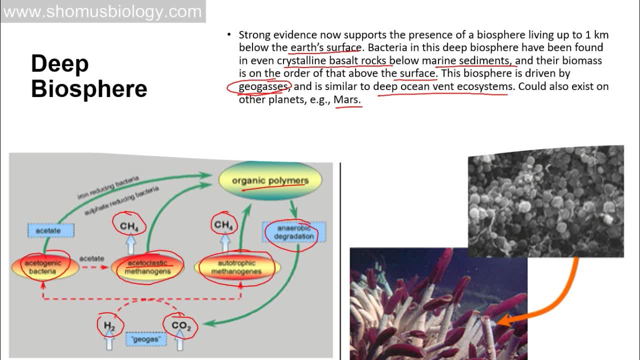 organic polymer. and again, this organic polymer can be an aerobically degraded and they can produce a CO2 hydrogen again. Okay, so this process continues. Acetogenic bacteria can produce acetate and is acetate Can be utilized by Iron. 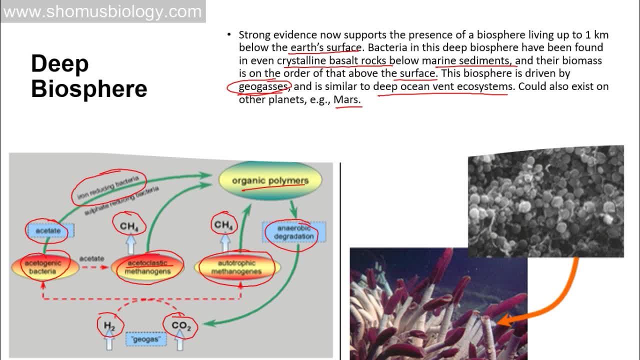 Reducing bacteria, and they can also produce organic polymer, and again, the process of degrading organic polymer into hydrogen carbon dioxide continues. Okay, so this is how deep biosphere functions. You can see, a bacteria does not require any solid nutrients to leave and survive. 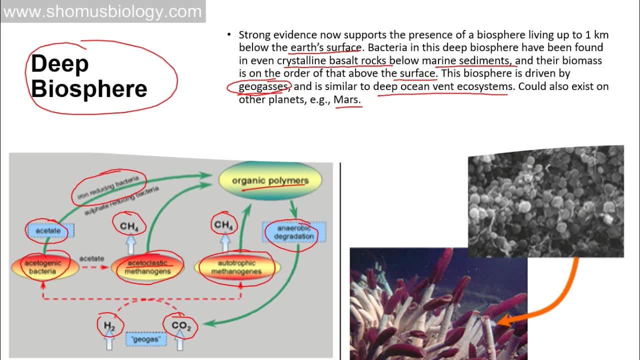 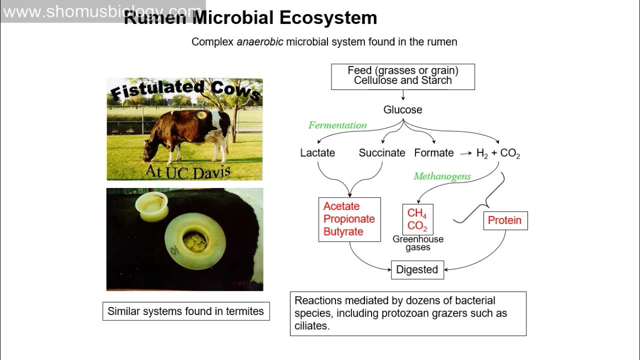 They only need the gaseous environment, hydrogen carbon dioxide, done. They can utilize them and they can produce is positive feedback loop, utilizing them vigorously and producing energy. For example, you talk about this same type of environment there in rumen of of cow microbial. 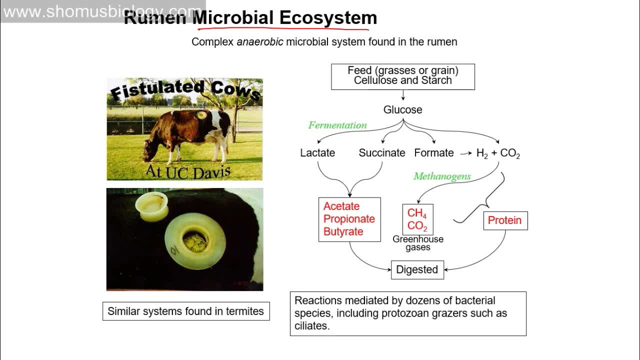 ecosystem in the rumen complex anaerobic microbial system found in this room and, as you can see, this is a cow and actually there is a literally a hole in the stomach of the. how you can see, this is the whole. Okay, All in the stomach. 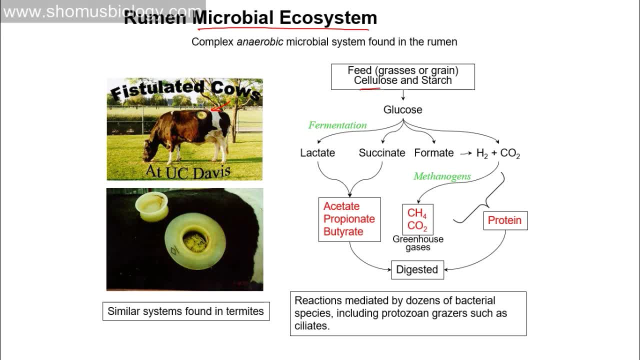 Now We feed them with the grasses or grains which contain cellulose and cellulose. Now we feed them with grasses or grains which contain cellulose and cellulose. Now we feed them with grasses or grains which contain cellulose and cellulose. 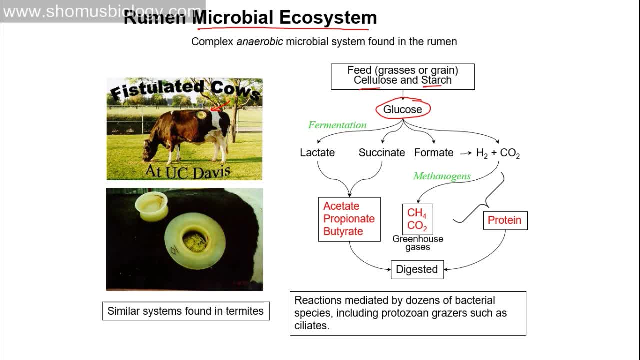 They also НАG and starch. it is converted to glucose, then a fermentation of glucose produce lactate, succinate, formate and all on. that can be degraded into hydrogen carbon dioxide which is used by methanogen. that is leaving in the rumen, in the gut of the cow. 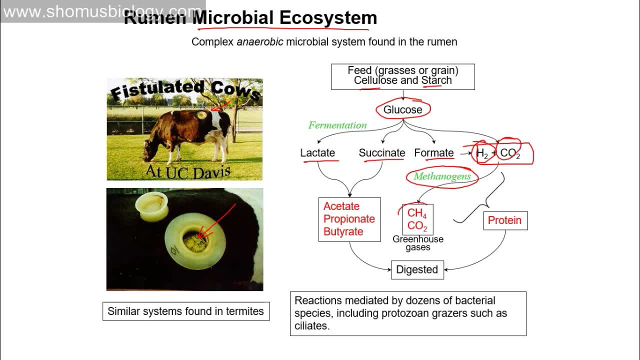 and the intelligent. so there take the hydrogen carbon dioxide as a gaston, produce methyl and carbon dioxide, which both add greenhouse gases and that can be reduced out Okay. succinate can can produce acetate, propionate, butyrate and they can be digested okay by the. 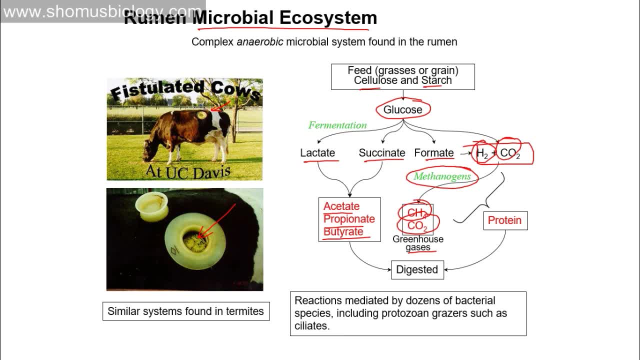 cow itself? okay so, reactions mediated by dozens of bacterial species, including protozoan such as ciliates? okay so this similar systems are also found in termites, but in a little different manner. the chemical process remains the same, but the way it works and the locations are different. 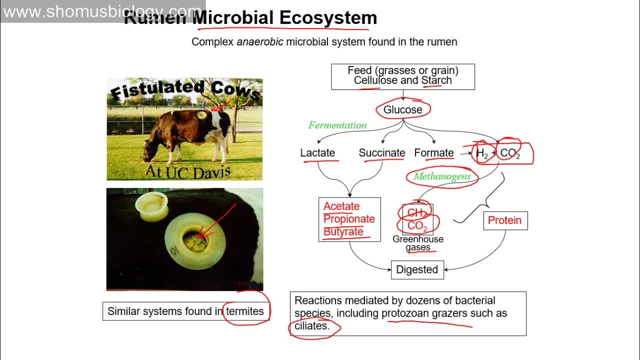 so in cow we can create this, like we can literally drill a hole through the stomach and we can insert this, this methanogens, there. we can utilize this hydrogen and carbon dioxide gas and produce ch4 and co2 and we can release it outside so they help in the digestion of the cow and that helps. 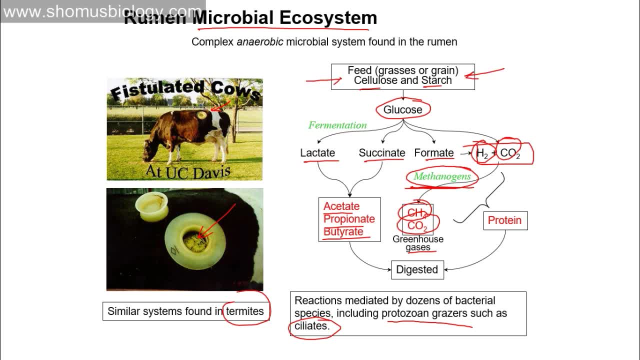 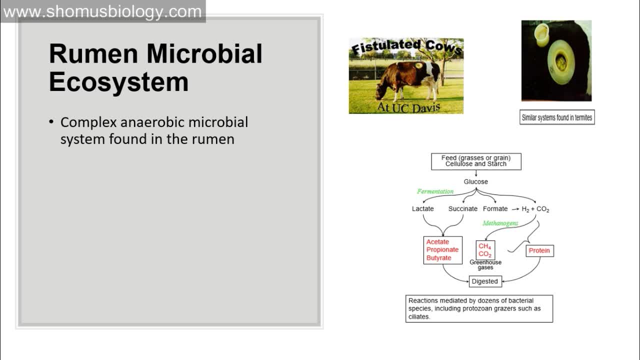 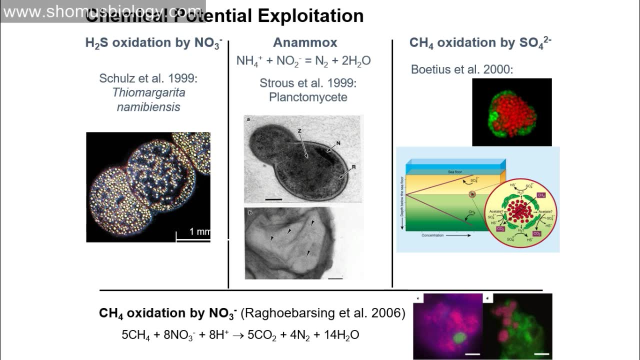 so, so, so. so think about all the situations where hydrogens sulfide is oxidized by nitrate and there and amok situation and ammonium is again interacting with nitrite to produce nitrogen. an nitrogen can be leasing to the air as free nitrogen source. this is like ammonia nitrogen. 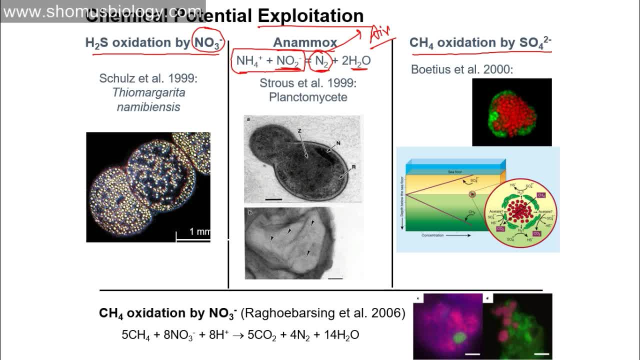 can be assimilated into the soil of the moon- nitrogen assimilation. so they also another process of removal of nitrogen into the air, and that is an amox, it's a, it's a two-step, it's a one-step process, jumping two different steps: of ammonium, like nitrogen assimilation, like methane oxidation. 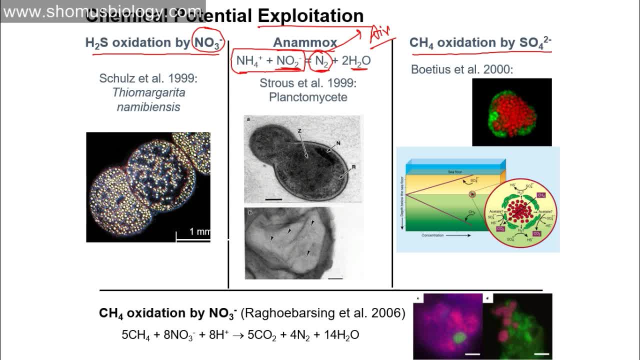 by sulfate again can be done by the bacteria. so the different research papers are listed here. who found out the different discoveries, particularly 1999 and 2000, and the methane oxidation by nitrate. you can see how exactly methane oxidation is done by nitrate, so particularly. 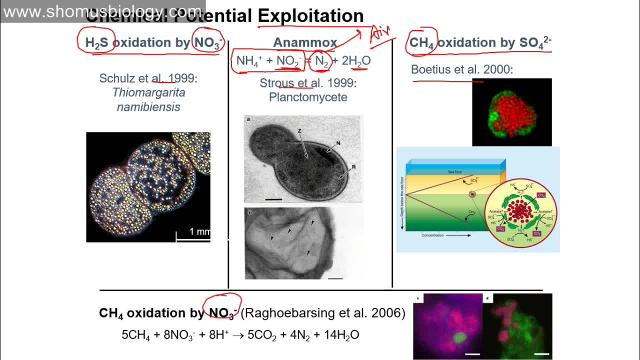 methane or hydrogen sulfide can be oxidized by nitrate. ammonium can be oxidized by nitrite and methane can also be oxidized by sulfate. so nitrate, nitrite, sulfate- these are the oxidizing agents who can oxidize harmful components like hydrogen sulfide, methane, and they can 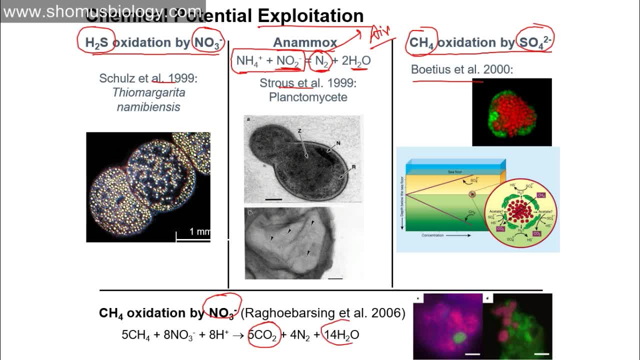 produce. ultimately, they can produce carbon dioxide gas, water and nitrogen gas and they have hydrogen gas. so you know, in in environment, the microbes play a vital role in converting up methane or ammonium into, like hydrogen sulfide, into less toxic gaseous components like carbon dioxide, nitrogen, hydrogen water, those things. so this is the the the feature. 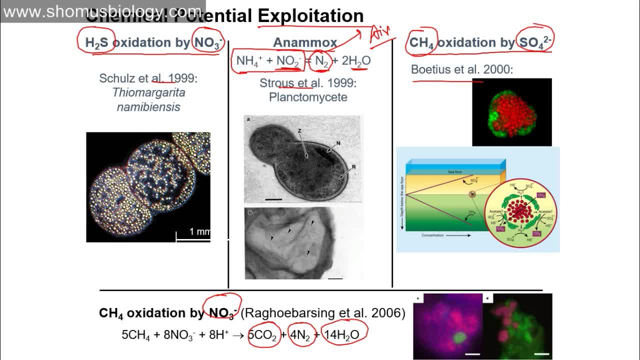 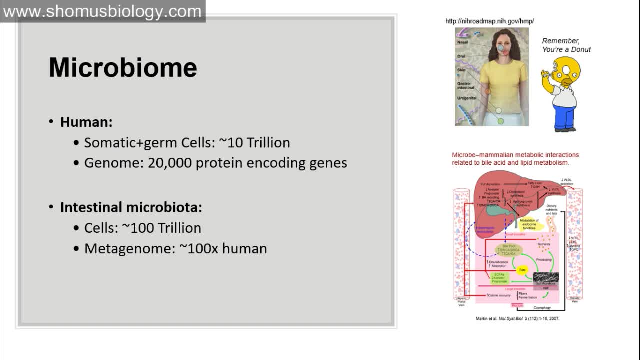 by different chemical measurements they converted and mostly of this process that oxidation and oxidizing agents are nitrate, Nitrate, Microbiome, human. if you think about the somatic and germ cells, near about 10 trillion microbes are found and you know the genome: 20,000 protein encoding genes are present. and if you think, 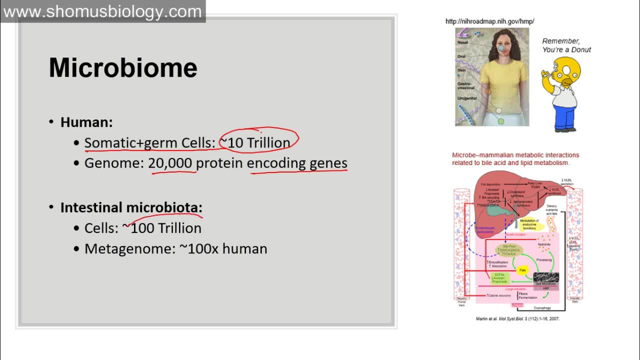 about the intestinal microbiota, the cells: 100 trillion somatic and germ cells in human body is 10 trillion 20,000 protein coding genes, while if you think about the microorganisms present in our body, our own cells are 10 trillion only, while intestinal microbiota is 100 trillion, which is 10 times. 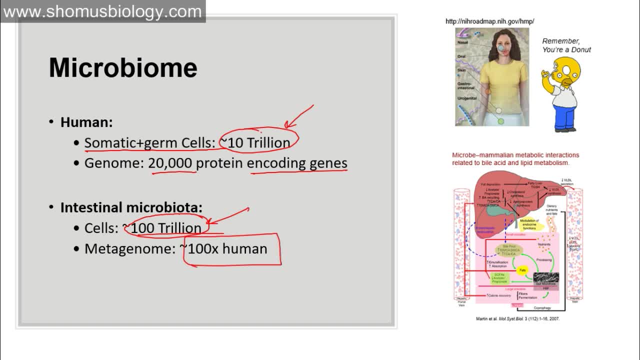 that up. I mean 100 times in this case is same, since 10 times of the total cells, and metagenome is almost 100 times than the human genome of the body. so think about it. so the microbiota that is found in our body. 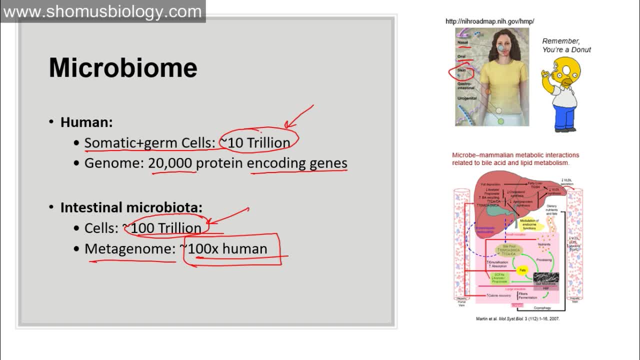 Starting from the nasal cavity, oral cavity, skin, gastrointestinal region, urogenital region. these are the components. the maximum is found in the gastrointestinal place, where we have 100 trillion cells of microbes, which is 10 times greater than the total number of cells found in our body, and then there are almost a microorganism: skin, urogenital tract, oral. 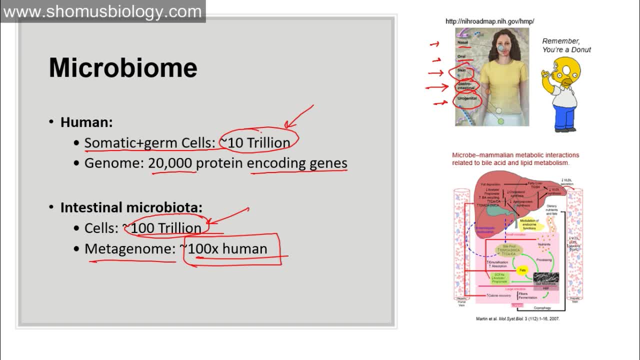 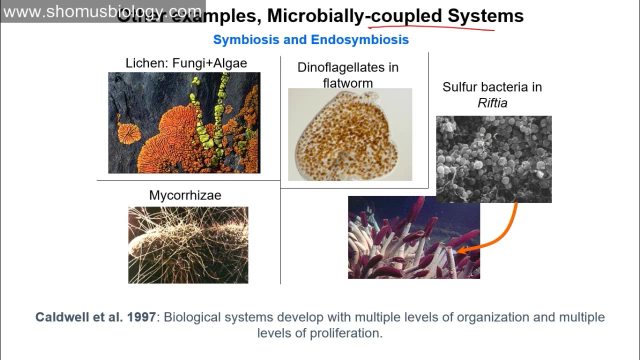 and nasal cavity. Got it Okay, Okay, Okay, Okay, Okay, Okay, Okay, Good to know, Thank you. So first thing I wanted to share with you is the results of microbial e coupled systems, where you find out that in our body. 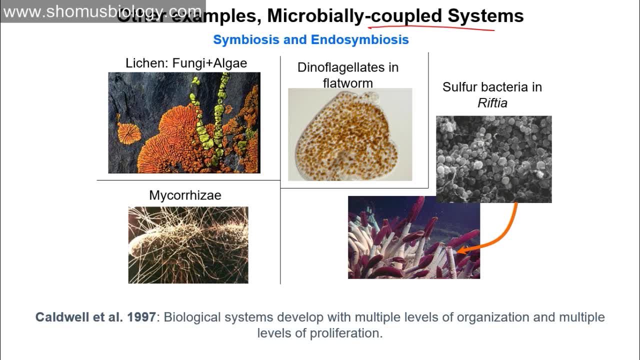 Also you can see in interesting microbes are present and this interaction in symbiotic and this interaction is beneficial, like mutual understanding between the microorganisms living there and us, because microbes get nutrients from us and instead Michael's also got an Arabic environment sometimes and in return, 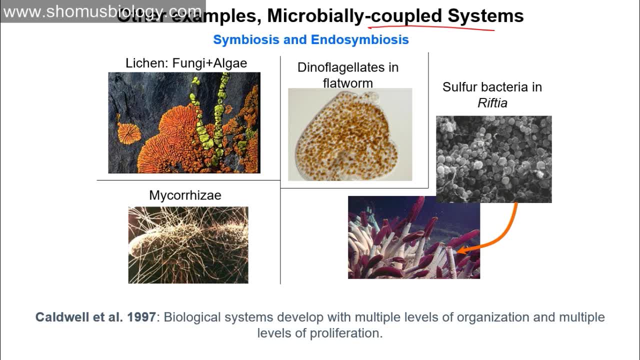 What we get is that this microorganisms present there, They produce vitamin uh, they help in our uh proper absorption of the food. they help in in the digestion a little bit and, the most importantly, they help in producing a strong immunity there so that some pathogen 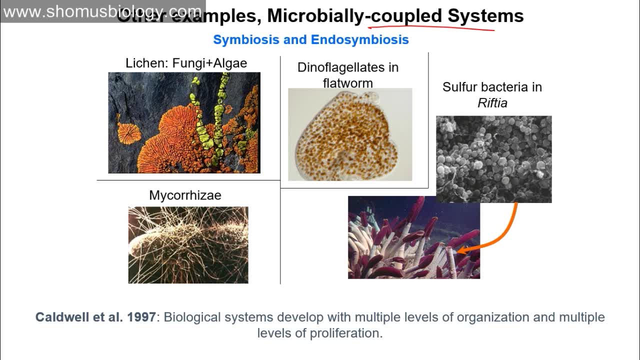 cannot colonize there easily. they will prevent foreign pathogen colonization in our intestine and they protect us against different intestinal diseases. now the situation is: if we remove all the intestinal micro flora of our body, then ultimately we will feel more sick for the intestinal diseases and different infections- pathogen infections like salmonellosis as well. 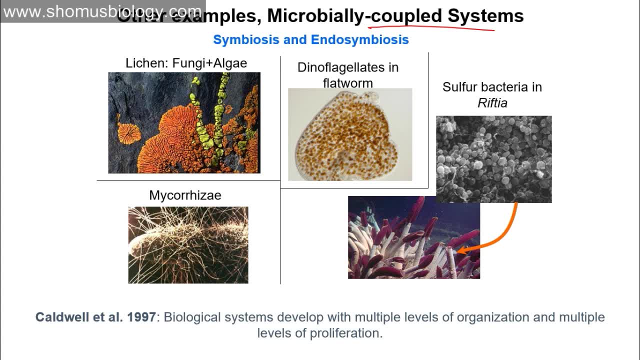 as you know, different toxin mediated diseases, diarrhea and all these diseases quite often so this intestinal microbiota protects us against this. so, apart from the intestines, if you think about the, the interactions between between this, uh, other microbiota and this micro in microbial interaction, then will find this like, in which is also some. 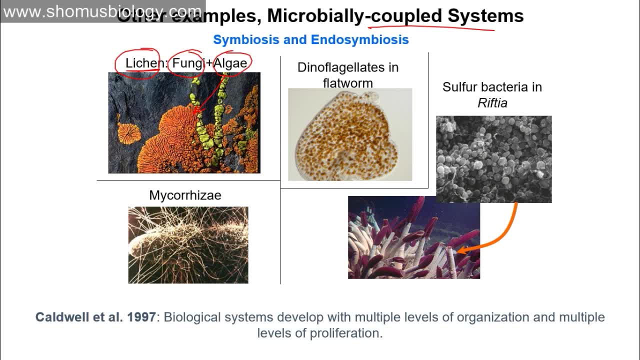 by details in between the fungi and algae living together with these gorgeous uh color dino flagellates inside of platform. so this is a flat form you can see inside the platform. belly is filled with small dino flagellates which live together in factors- huge number. 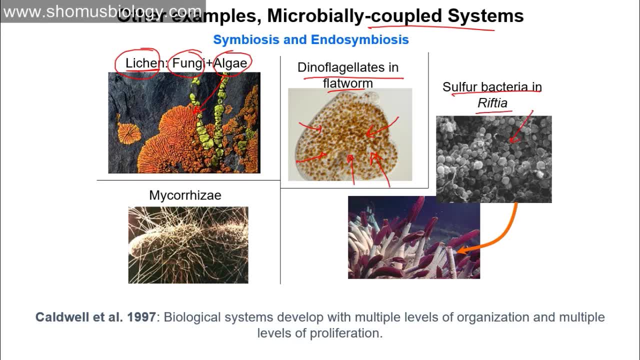 sulfur bacteria in riftia. they present together. to look at the riftia, this is the coral-like structure, structures underwater, sulfur bacteria present there and mycorrhizal, which provides essential benefits to plants, and particularly you know. that's the reason we produce mycorrhizal culture. 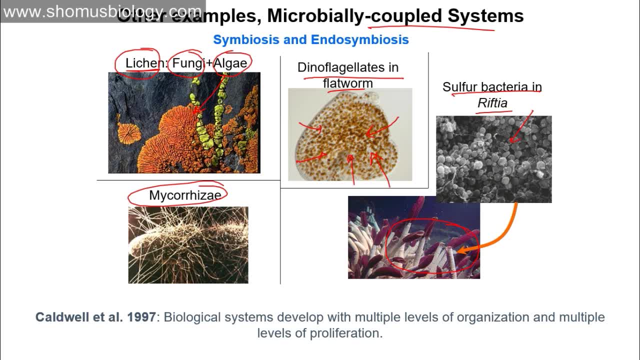 separately and people add that into the soil when the plant trees. so the plant can take up nutrients properly and they can fix the nitrogen quite well and can utilize the nitrate ammonium from the soil properly. Okay, so these are the different types of interactions. 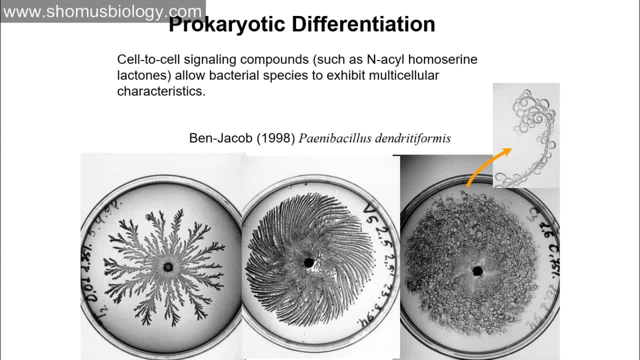 that are found in the nature. apart from the human body, prokaryotic differentiation, cell to cell signaling compounds are present, such as in acetyl homoserine lactones. They allow bacterial species to exhibit multicellular characteristics, and this is very, very important. to understand the multicellular characteristics of a bacteria, you know particularly when. 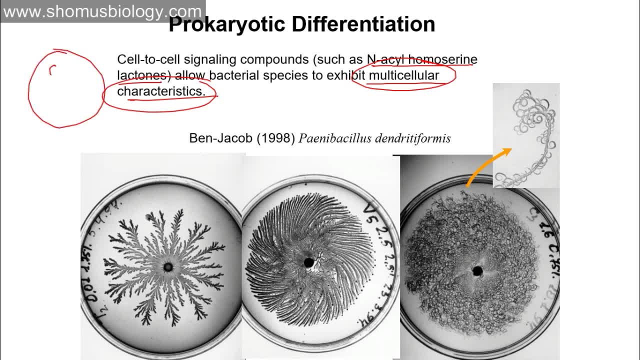 we see the bacterial culture, bacterial colony, will find out. it's of a particular shape. Sometimes it can be smooth, Sometimes it can be. It looks like like you can see in this picture their different shape If you look at your. so different species and different type of microorganism colonize differently in the 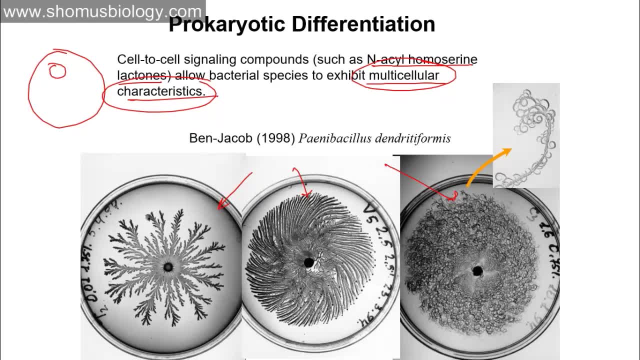 in the agar plate, because they have a particular way of arranging themselves to one another, attaching themselves to one another. It's always true that one particular microorganism is not enough to cause any disease and not enough to colonize itself, so they need help from other. 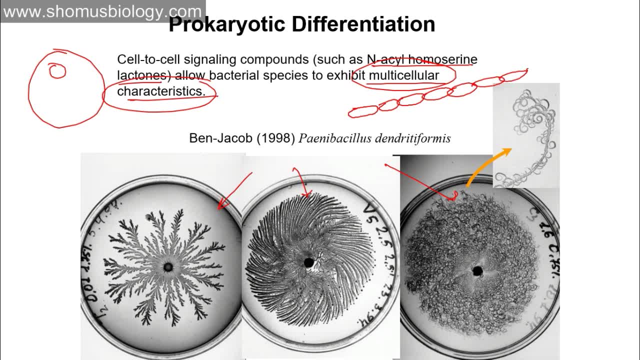 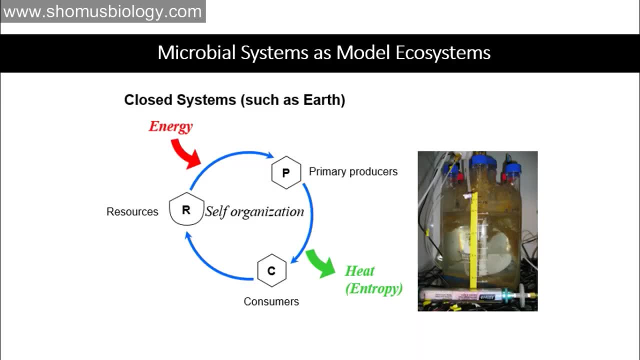 They need to be able to do it because their own members to link properly. some of the manager like a change of the manager is like a stacked. some of the managers like a layer and that's how the form of the tissue layer. so microbial systems are used as a model system. closed. 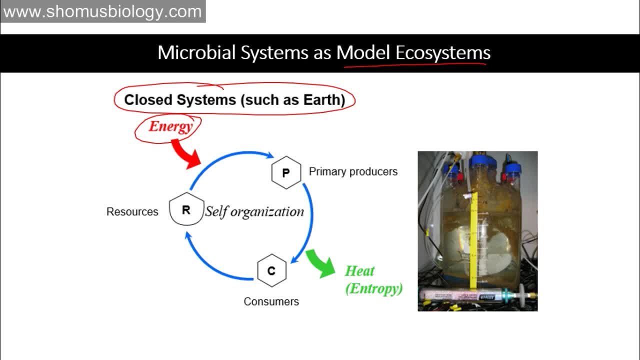 system such as earth. to think about it, energies are the key to drive the system's energy is present. primary producers take up the energy and producers are producing food and consumers are taking up this, this food. consumers are taking up the food and, by this means of food production, they produce heat. 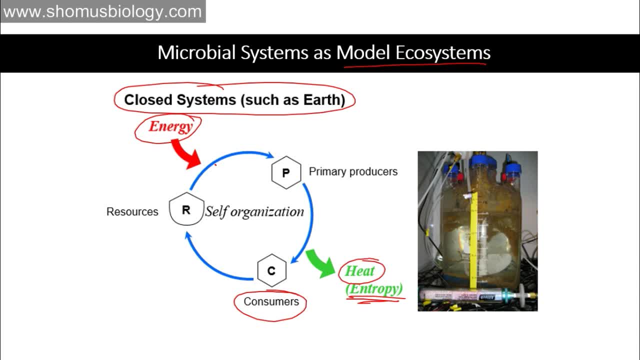 that is, entropic. chaos is increasing outside and consumers started in. the primary producers and consumers are also producing few resources for self-organization and is some resources, particularly like CO2, H2O, hydrogen nitrogen in some occasions. These are few occasions but CO2 and H2O, So this components are used by the primary producers along with energy. 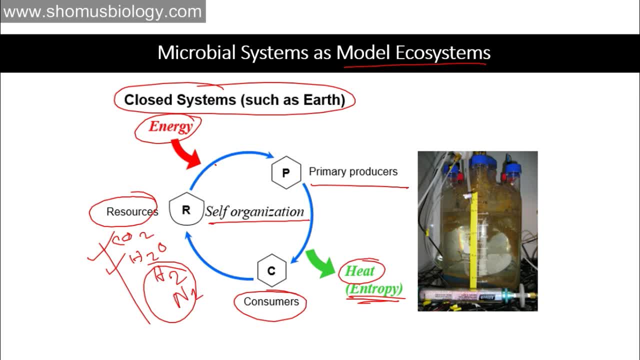 to produce food. So you know, when we discuss about the primary producer and consumer, we always say that consumer are dependent on primary producers. but if you look at this picture you get a sense that the primary producers are somehow indirectly get some. 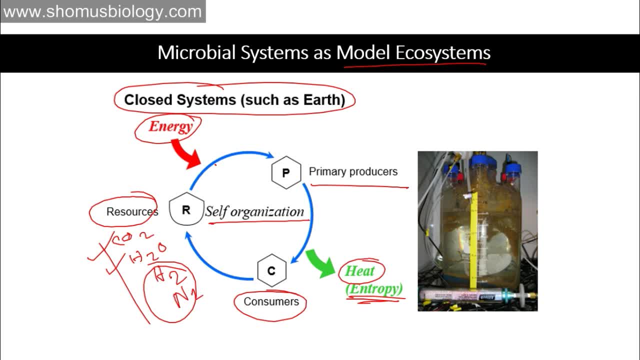 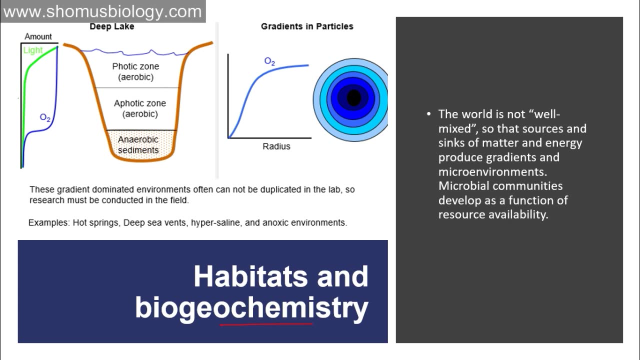 benefit from the consumer itself, because the consumer are producing some sort of resources, like CO2 and water, that can be utilized by by the primary producers. Okay, So habitats and biogeochemistry- The world is not well mixed, as we know, so that sources 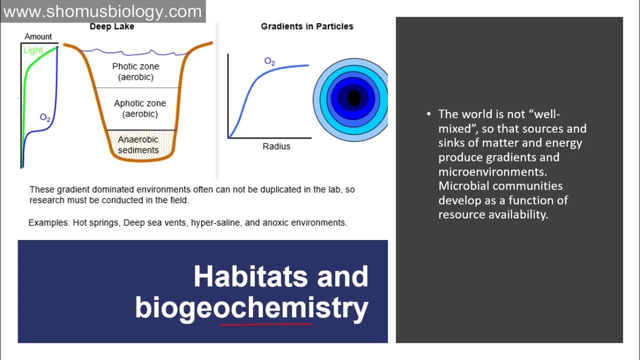 and sinks of matter and energy produce gradients and microenvironments. microbial communities develop as a function of resource availability. So think about it. If you look at here that in deep lake and as well as in gradients, in particles, think about the differences in the deep lake. You can see there are different zones: four tick zone a. four tick zone a. 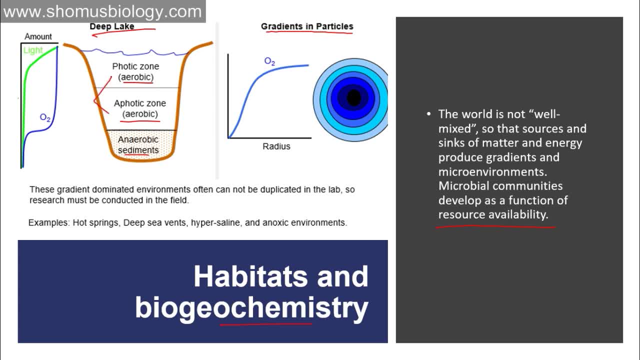 four tick zone and Arabic sediments. four tick zones are Arabic, both four tick as well as a four tick zone, but the difference between four tick and a four tick is that four tick zone receives maximum sunlight. That's why 40 a four tick means they don't receive that. 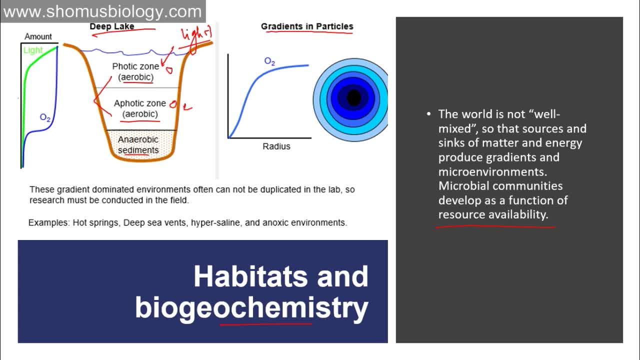 much of sunlight but both are Arabic, so they they are exposed to oxygen properly. Okay, so light concentration, you can say the availability of the right, the amount of light available, both in 40 can afford a zone are different. Okay, in 40, it's very less. in a 40 you can see the, the decrease. it's very less in a 40, but the 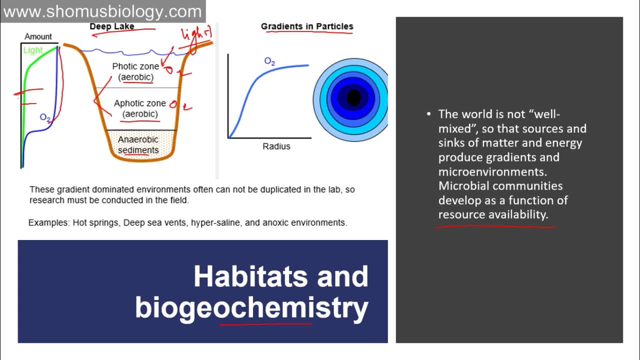 oxygen availability is almost the same present in 40 and a 40 zone. this all oxygen is well available, but from the anaerobic sediments you see, the oxygen concentration is decreased suddenly. and the anaerobic sediment, as it's a sediment, it's not the water layer, it is. 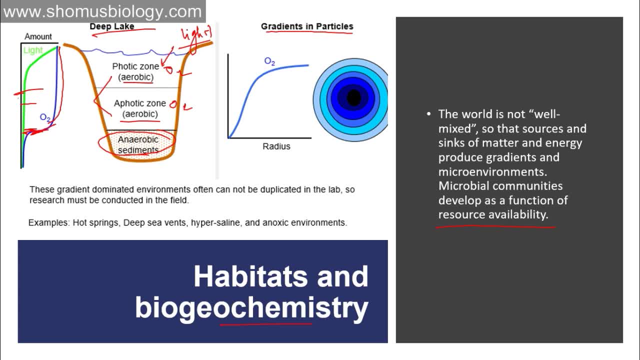 sediment made up with soil, clay and other rock components. so here the oxygen concentration decrease uh dramatically. it's an anaerobic condition. example of this: hot spring: deep sea vents, hypersaline and anoxic environments. you can see, and not only it's about the fatigue. 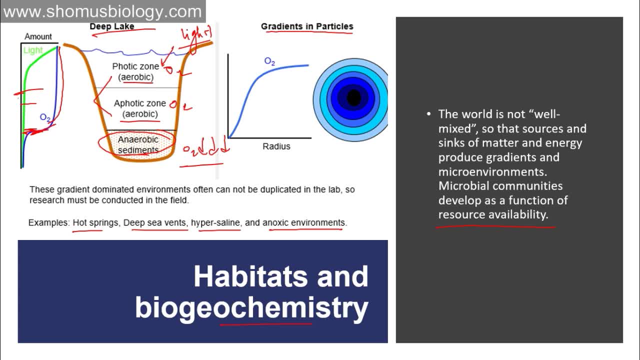 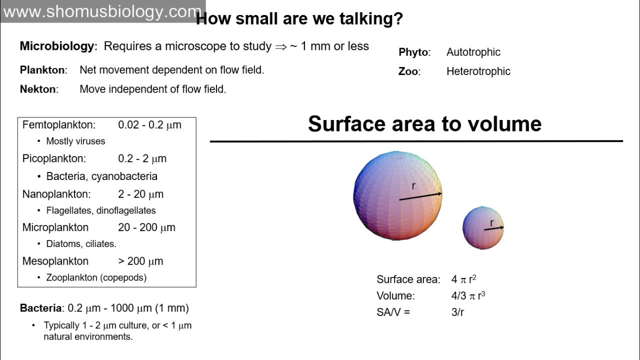 and oxygen's availability. think about the oxygen's availability in the radius. it also oxygen is available based on the radius systems as well. so the radius: as we are going down, the radius, the oxygen availability getting less and less. it's available more in the outside, surrounding radius. Now, when we are talking about the microbial ecosystem and talk about 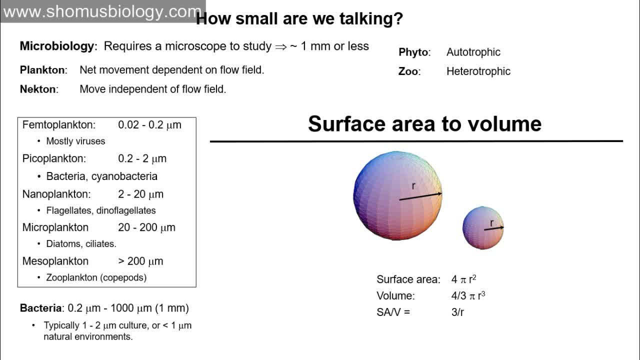 microorganisms. we're talking about small things, miniature things. So how small we are thinking microbiology requires a microscope to study. we all know that the planktons are the primary producing the aquatic environment, So particularly their phytoplankton, zooplankton. phytoplankton are autotrophic. They are the producers. Phototrophic means they will, autotrophic means they are. they are capable of producing their own food And they utilize energy directly from sun. So they are phototropic, photoautotropic, and zooplankton are there, which are heterotropic. 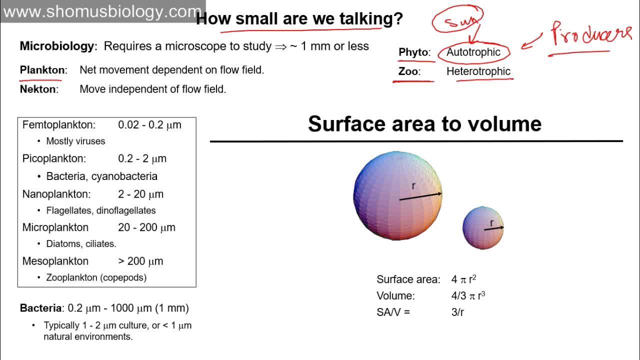 That means they don't utilize the sun's energy directly. they they utilize other chemical sources and energy sources, other chemicals, as an energy source to use it. So femtoplankton are very, very small- is the smallest, So they are mostly viruses- 0.02. 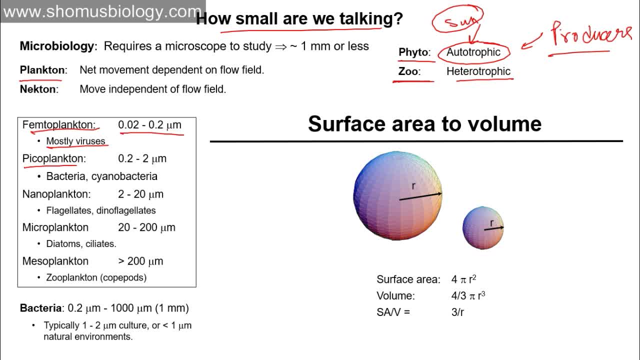 to 0.2 micrometer. picoplankton, 0.2 to 2 micrometer. bacteria, cyanobacteria, nanoplankton. two to 20 micrometer, which are flagellates and dianoflagellates, microplankton, example diatoms and ciliates. 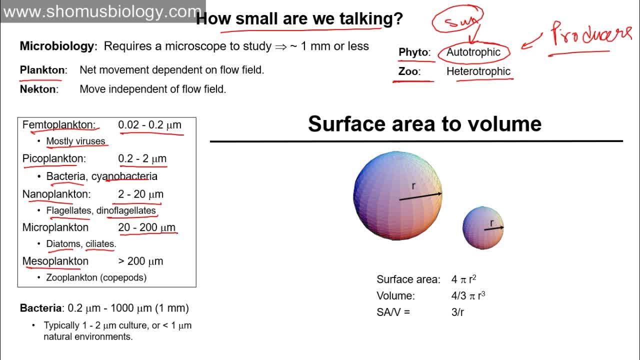 20 to 200 micrometer and mesoplankton. example: zooplankton, copods, greater than 200 micrometer, Dierton. So zooplankton, mesoplankton, which are much bigger than the phytoplankton animal, phytoplankton f, adult plankton, picoplankton, nano plankton, microplankton. So think about. 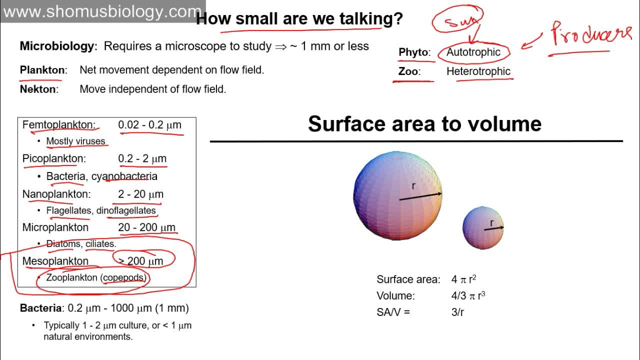 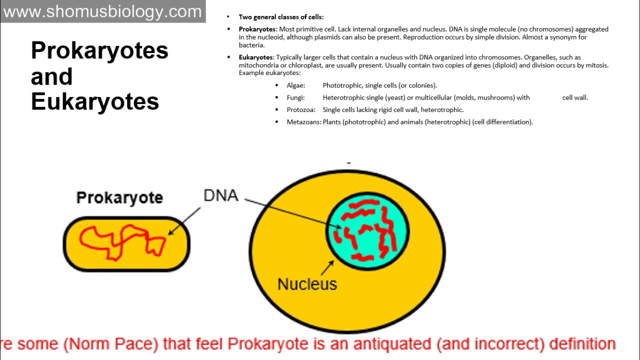 here. maybe we talk about the year we are talking about. we're talking about the dimensional kit. So what? we buatchkn all these in the ecosystem. We had two Same size nat beauty plants were types of cell prokaryotes and eukaryotes, and we know about the differences between. 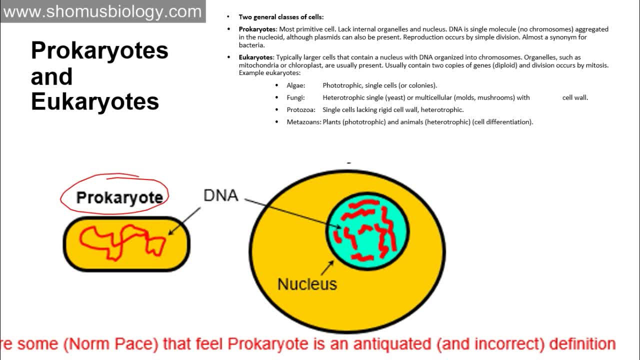 prokaryotes. in a quite, quite well, prokaryotes and eukaryotes. The major difference is that in eukaryotes we have membrane bound organelles, while in prokaryotes we don't have any membrane. 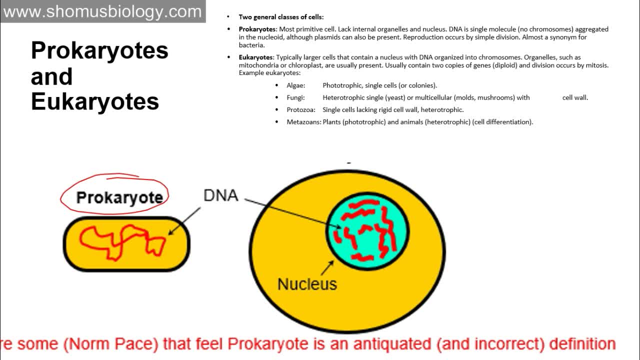 bound organelles. So in eukaryotes, larger cells that contain nucleus with DNA organized into chromosomes- okay, and organs like mitochondria chloroplasts are usually present. So the examples of different eukaryotes: algae, fungi, protozoa, Mesozoa, metazoa, LG, phototropic- they can. 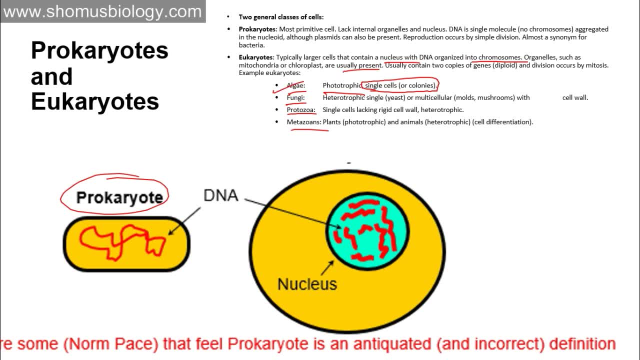 be single cells or can be present in colonies, fungite haterotrophic single cells like yeast, or multicellular, like molds and mushrooms, and they have cell wall. This is the unique feature about fungi protozoa- the single cells lacking rigid cell wall, and they also 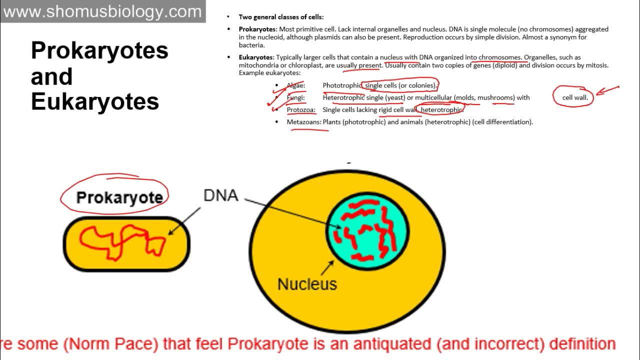 are heterotropic, So fungi and protozoa both depends on the, The other autotrophs for their food, Metas ones like plants and animals. among plant plants are phototropic because they can produce their own food. Animals, hydrotropic, cannot produce. 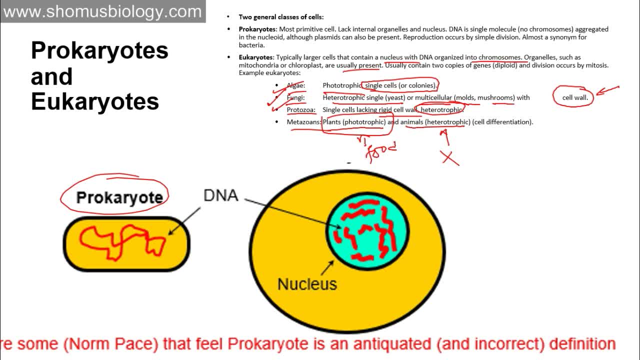 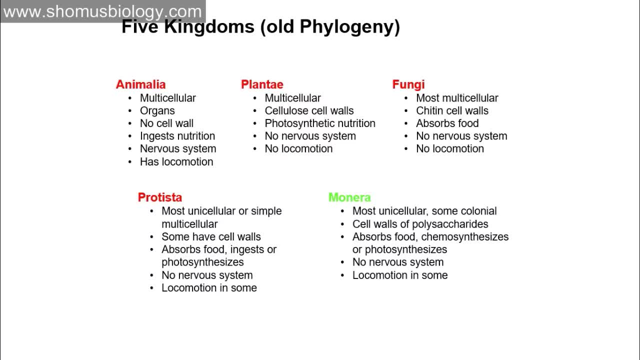 their own food And the difference between plants and animals are plenty, but we know that animals have a cell differentiation and specific cells of specific functions. So the five Kingdom concepts for old phylogeny utilizes this concept. Now we only talk about three domain concept. Okay, I mean, you carry up bacteria and archaea, We'll talk about that. 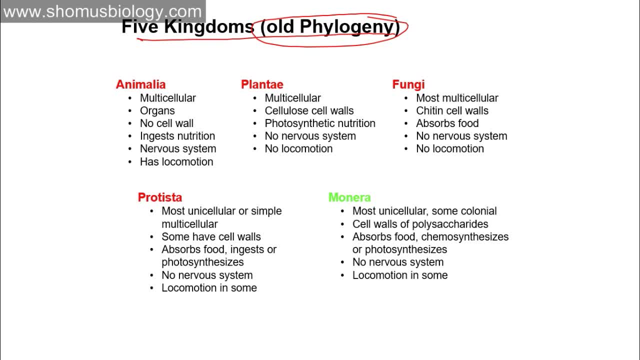 in a moment, But earlier times. we are old phylogeny where five Kingdom concept are famous, like animalia, plant, fungi, protist and monera. When animal in a male's multicellular contains organ, no cell wall ingest nutrition, nervous system and locomotion is present. planty multicellular. 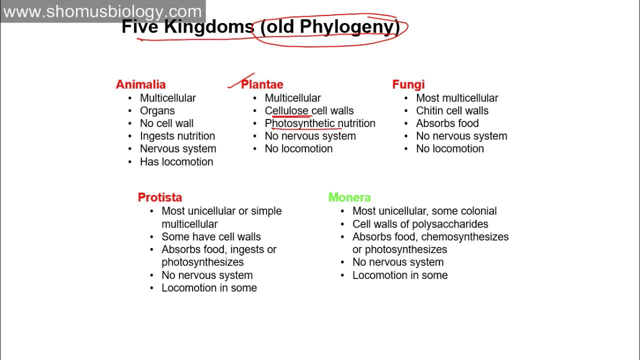 cellulose is present in the cell wall, photosynthetic, no nervous system, no locomotion, Which is differing plenty from animalia. fungi, mostly multicellular. the cell wall contains kiting. It absorbs food, no nervous system, no locomotion, and fungi can also become a. 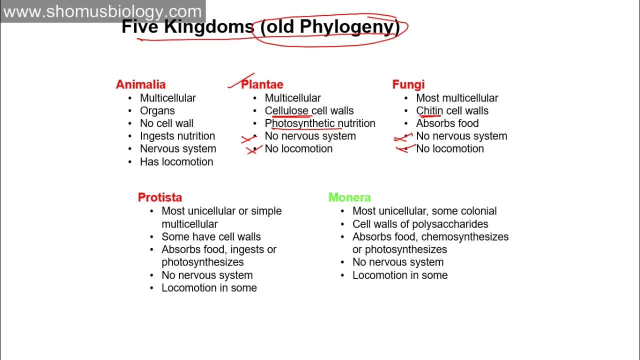 kind of you know decomposers protista, mostly unicellular or simple multicellular. mostly are said unicellular means made up with one cell. Few are present with multiple cells. Some have cell walls. They can absorb food, ingest and photosynthesize. 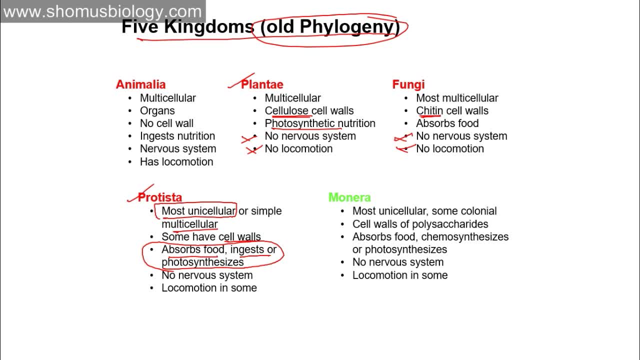 So everything is possible by protista, because protista is a mixed group. they don't have any nervous system, but some of them has locomotion monera, mostly unicellular. Some are colonial means. they produce colony. cell walls are produced by photo. I mean polysaccharides. 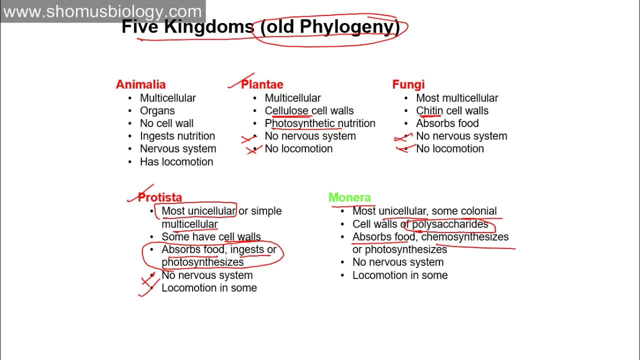 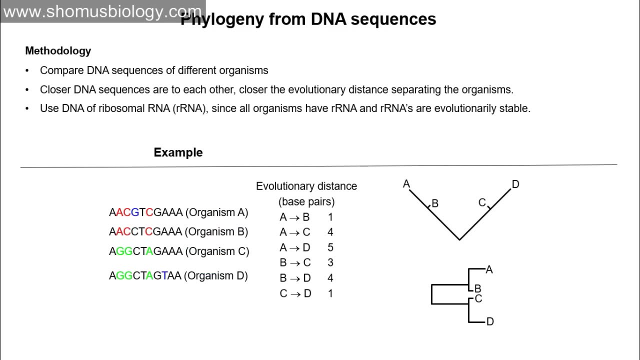 it absorb food. chemo synthesizes means they take energy from chemical. I mean they take the carbon source from chemicals and they can also sometimes photosynthesize. no nervous locomotion is found in some of the monera phylogeny from DNA sequences. now, 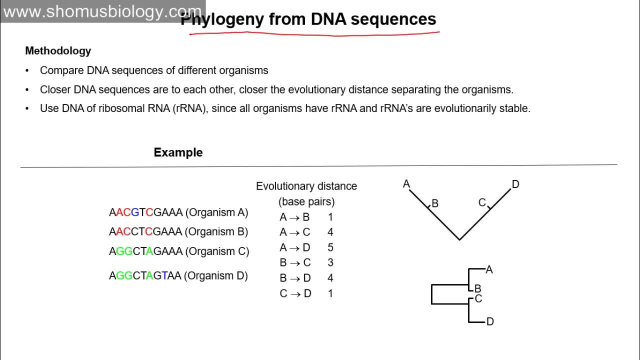 there are modern methods to be used in the phylogeny analysis and the methodology is to compare DNA sequences of different organisms, because we sequence them and then we compare the DNA sequences. we can compare them because we have- we have the databases with the DNA sequence, a complete DNA. 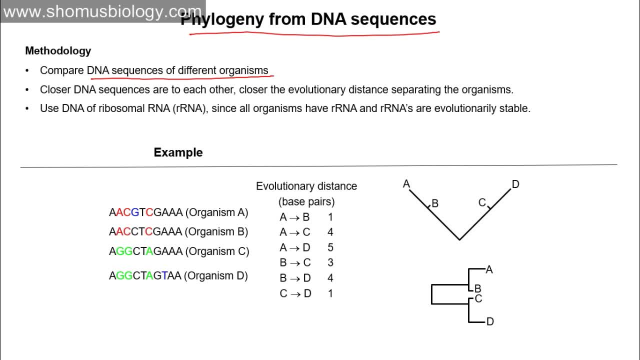 sequence of different organisms and compare them online in the database. when you run blast with bioinformatics we get to know the similarity score between two organisms. okay to same organism has the hundred percent identical similarity and less than that means they have a little bit of difference. closer DNA sequences: 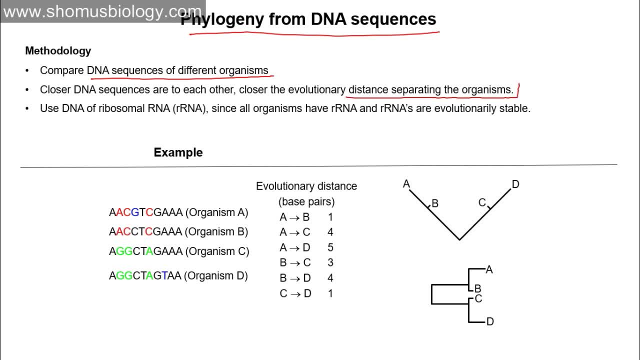 are to each other close at the evolutionary distance, separating the organisms, and use DNA of ribosomal RNA like our RNA. since all organisms of our RNA are RNAs, are evolutionary stable. our RNA have not changed much through the evolution time scale. that's why you use our RNAs okay to compare between the organisms, okay. so if you look at here, 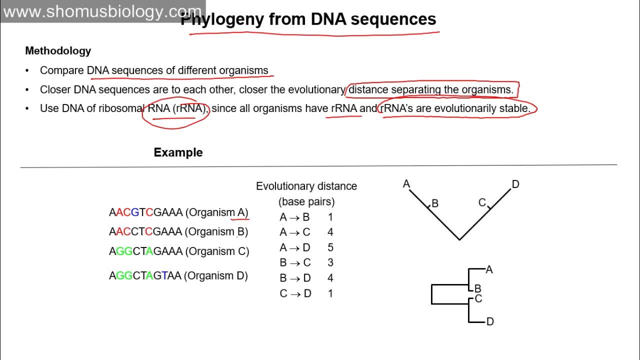 that the evolution distance. we are looking at different organism, organism ABCD, and we are checking the different similarity and differences. you can see that the difference here is between A and B is only once this G. this is the only place to to do to differ, rest, everything is same. so only difference is one, one base between A and C, if you. 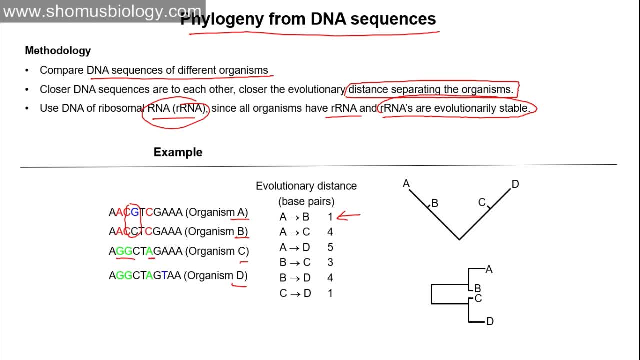 think about here this: three bases are different. so between A and C, we have one, two, three, three basis difference. between B and C, we also have three basis difference. between A and D. we have four bases. that are four places which are different. okay, are five places which are different, you can see. so this is how we can. we can. 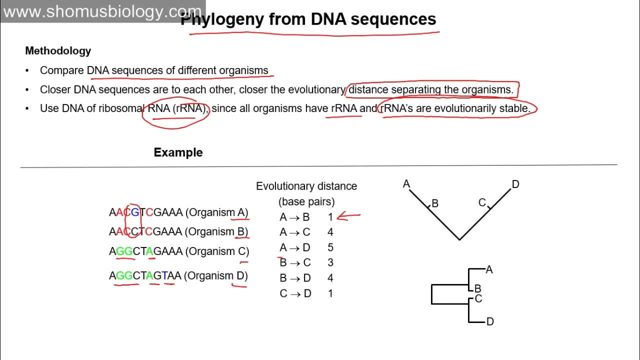 assume like by looking at this DNA sequences you can see that the least similarity is present between A and D, because five bases are different between A and D and are closest relative is A and B, and C and D. so think about it: A and B are closest relatives, nad and their distant most relatives. so A and B are 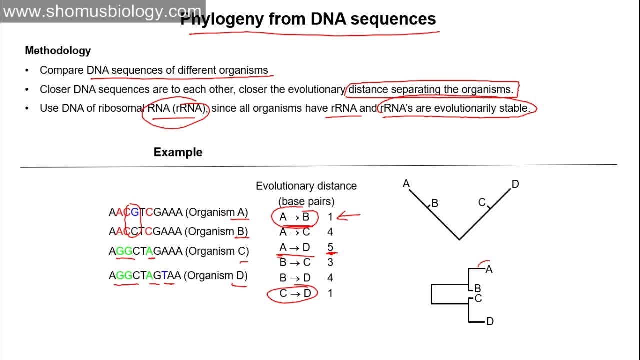 very close. that means they and B share a common base. so here there is one, two, three family between a and C and D. so what we are doing here here closed. that means A and B share a common ancestor. So A and B share a common ancestor. 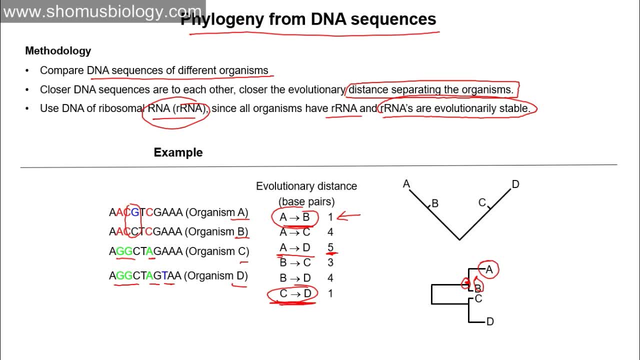 from where A and B branched. Similarly, C and D share a common ancestor from where C and D are branched, And now rest of the others are branched from a other common ancestor. So this will be the place. Okay, so A, B, C, D is done, And this is how it's placed. 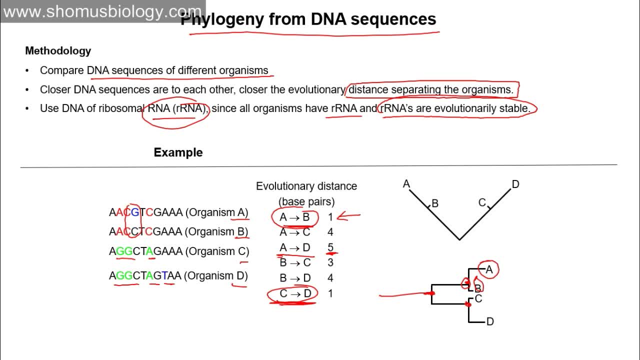 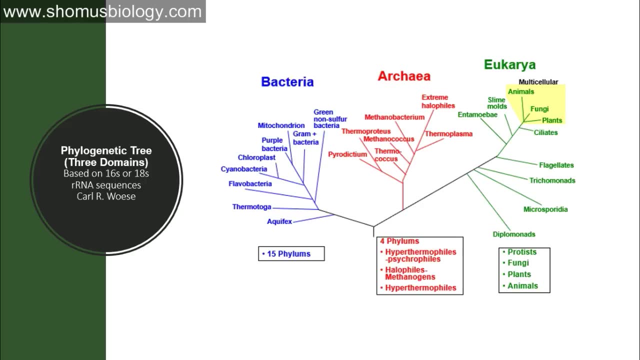 So this is how we produce the phylogenetic tree, And if you want to understand how exactly phylogenetic trees created and the methods to do that, you can watch the lecture in my channel regarding the phylogenetic tree analysis and how to do that. Okay, Now, in the modern 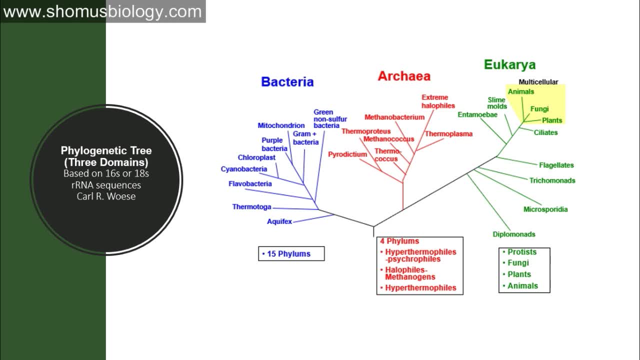 era. the phylogenetic tree that we have created in recent times, based on the, 16 is our RNA and 18 is our RNA sequence. Okay, and this system is brought by the car are ooze. So this system is known as three domain concept. 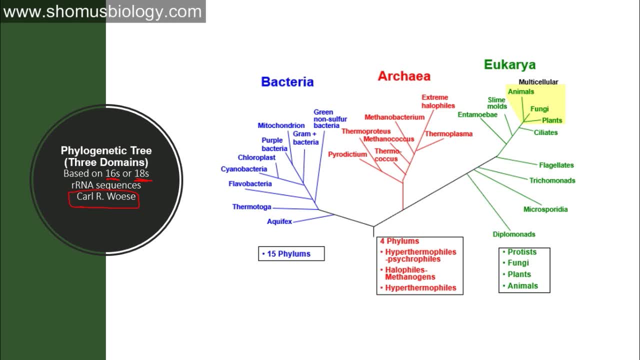 So every single organization has three domain concepts. So every single organization has three domain concepts. So every single organization has three domain concepts. So every single organism in planet can be divided into three domains. no big deal. no, 510 different regions, only three domains: bacteria, archaea, eukarya, that's all. Archaea are the primitive organisms. 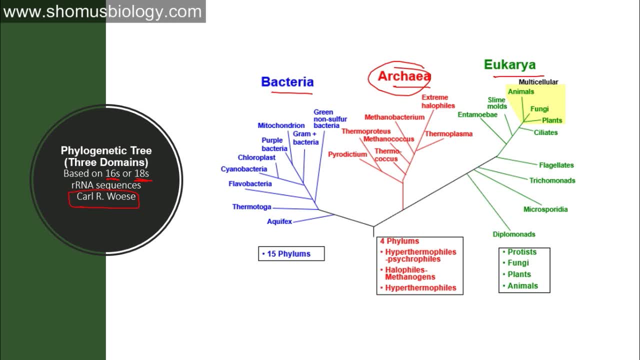 but they are mostly, you know they either hyperthermophiles or halophiles means they love to be present and survive in a thermophilic environments or halophilic environments. where the temperature is boiling hot or the the pH is very high or low, Archaea can survive. 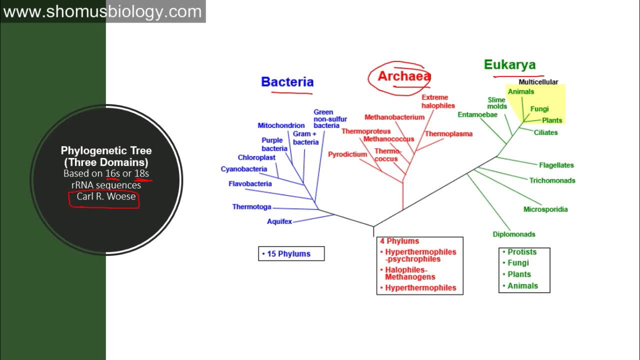 in this rough environmental conditions. So in most of the places where we found living creatures in very cold or very hot environments, they turn to be archaea. Then comes bacteria. Bacteria are present in every single locations. Okay, so they are also dynamic, ranging from 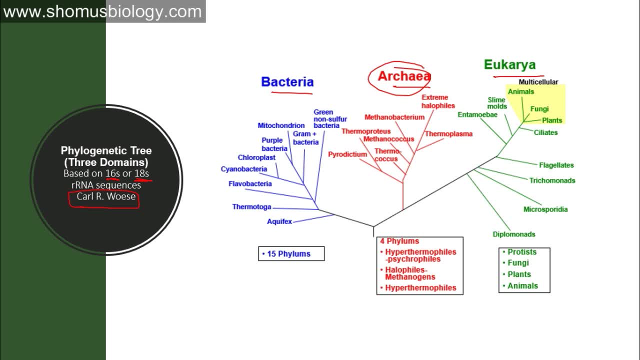 to five degrees Celsius, temperature till 60- 70 degrees Celsius, They can survive. And then there are eukarya, which are multicellular, and eukarya contains fungi, plants, ciliates, slime, molds, flagellates. Okay, so everything is present in the eukarya. 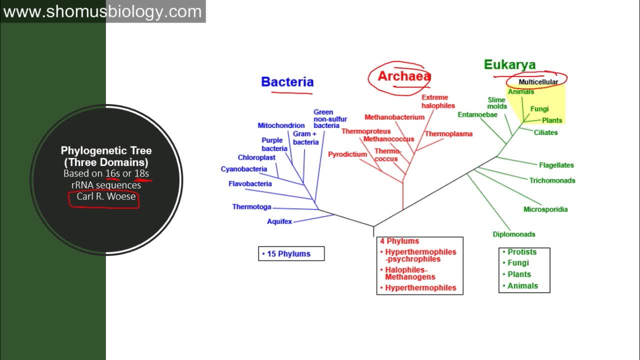 because eukarya in this case means multicellular, That's all okay, And bacteria means prokaryotes, and archaea is little different, Although archaea has more similarity with eukarya than the similarity with bacteria. So think about this picture: This is a common ancestor of: 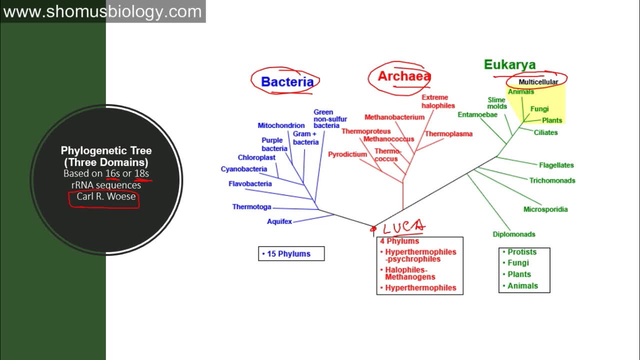 eukarya, We call them last unknown common ancestor, or Luka. Okay, a last universal common ancestor, Luka. From this common ancestor, one branch that produce bacteria at the beginning And then another branch continues After some time, there is another common ancestor and 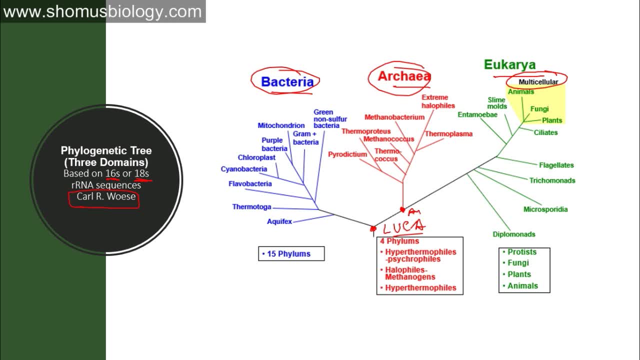 from this ancestor branch into archaea and another branch produce eukarya. So think that archaea and eukarya both share one common ancestor, while bacteria and archaea does not have that common ancestor sharing. So archaea and archaea have more similarity than the archaea has with bacteria. So in 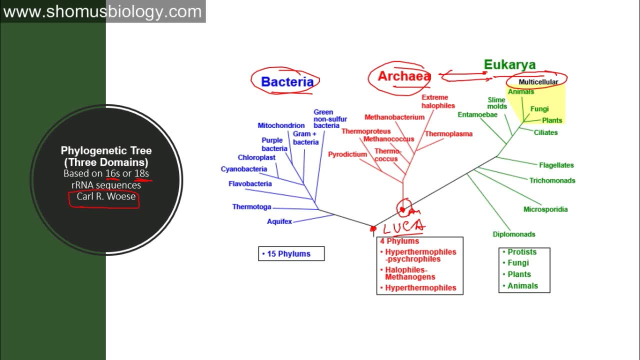 bacteria. there are 15 phylums. you can see all these phylums are listed: Aquiflex, Thermotoga, flavobacteria, cyanobacteria, chloroplast, purple bacteria, mitochondria, Bichem, apart because you know chloroplast and mitochondria, both are listed inside a bacteria because 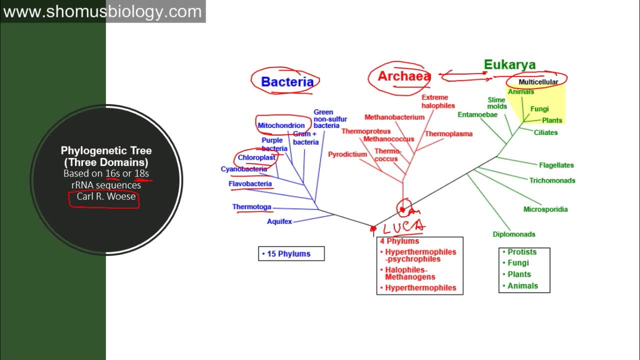 these are bacteria Which gets internalized into a eukaryotic Cell and then became the organelle inside the eukaryotes. but they actually are bacteria. They actually were bacteria. So we call it endosymbiotic theory, Then gram positive bacteria. 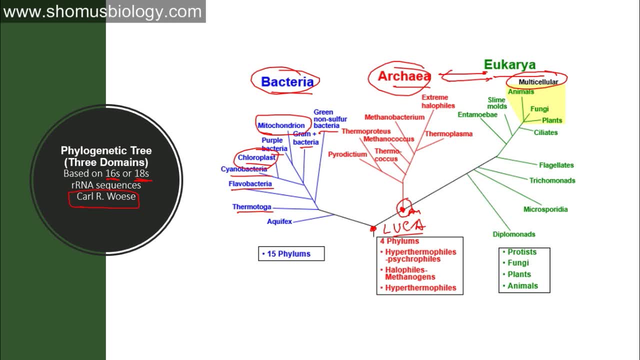 and then green non-sulfur bacteria came later In archaea. you can see different four phylums are present and those phylums are one type are hyperthermophiles, known as psychrophilic, halophiles, known as methanogens and hyperthermophiles. 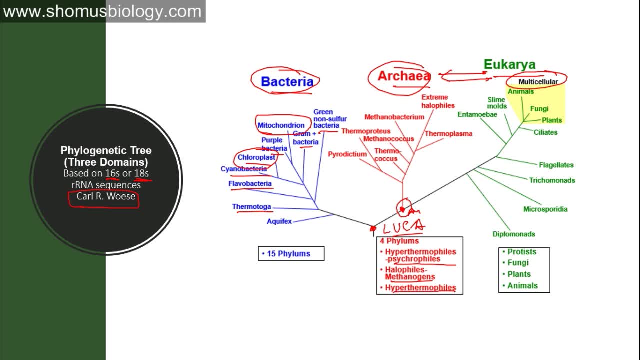 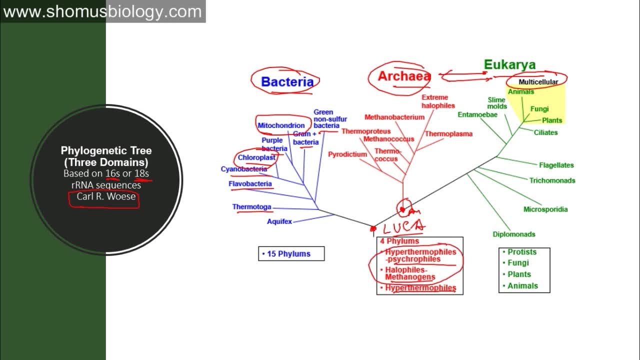 halophiles are the major type, but four phylums are present in this location. okay, Methano bacterium, extreme halophiles, thermoplasma, thermococcus, thermoproteus, methanococcus pyrodictium. So these are the examples of archaea Pyridicium type. 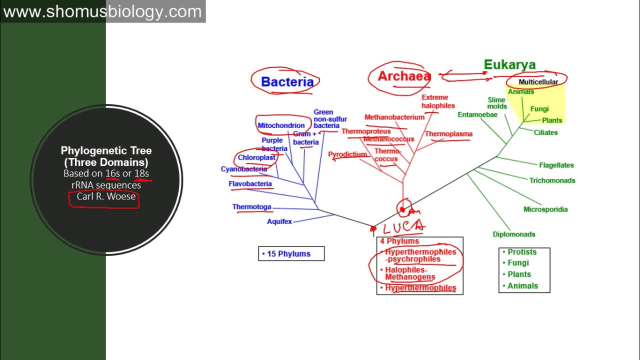 So these are all the different phylums, the types pyrodictium thermococcus, methanococcus thermoproteus, PS, Methanobacterium thermoplasma, extreme halophiles, okay, and you know by the name. 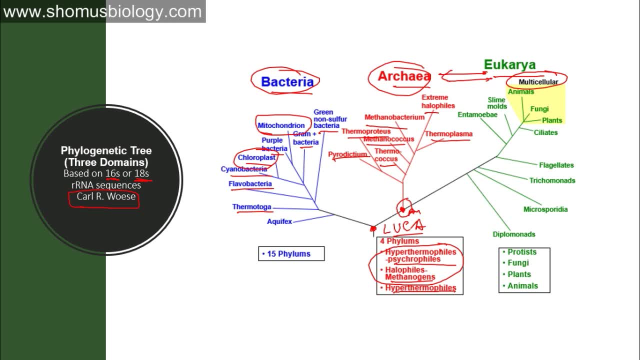 you can understand anything with the thermo name means they live in the very hot climate. halophiles live in a way in a- you know, changing osmolarity. okay, changing osmolarity is the place where the halophiles are present and also pH variations are there. they can also. 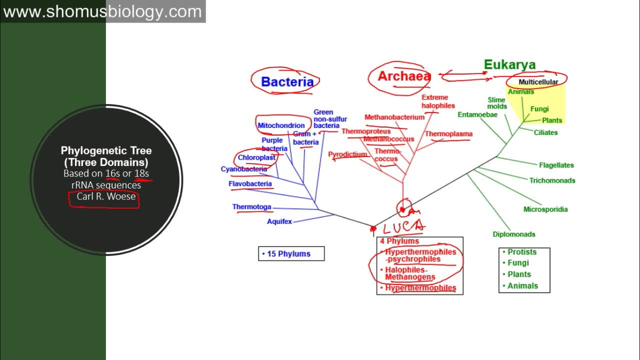 survive hugely pH variation and in eukaryotes you can see protease fungi, plants and animals are present in eukaryote. so in the five kingdom concept provided by Whittaker this protease fungi, plants, animal, all are placed inside eukaryote and then rest prokaryotes are made. 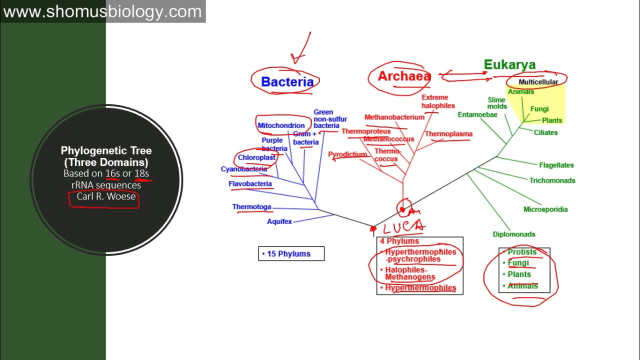 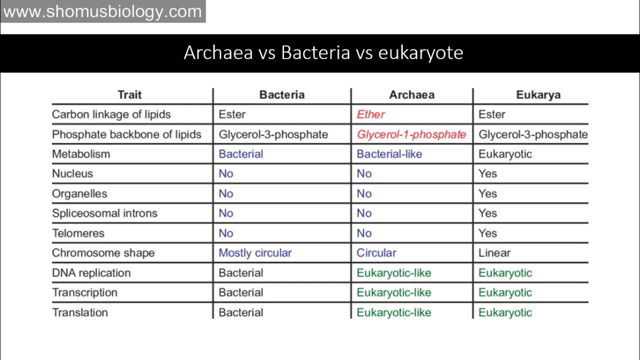 in a separate domain, bacteria, and the last and newly found domain became Archaea. okay, now the most important part, Okay, What CSN had great perspective is to know the difference between Archaea, Bacteria, Eukaryote. so think about the trait carbon linkage of lipids in bacteria. it's ester linked the hydrogen. 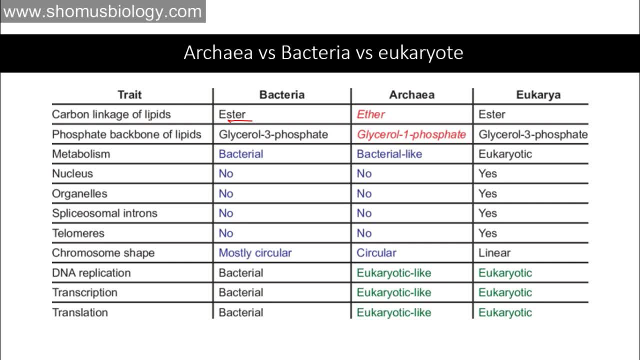 and carbon. you know the hydrocarbon chain linked with the glycerol backbone. okay, and this linkage in bacteria, it's ester linked in eukaryotes, also ester linked in Archaea, it's ether linked phosphate backbone of lipids. bacteria glycerol and glycerol are linked. 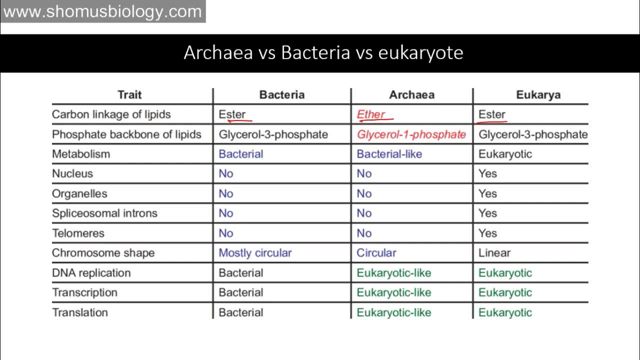 to the phosphate backbone and linites are linked with lipids in the phosphate backbone. so it was clear. these two traits, archaea, also glycerol, and Eukarya, and Eukarya also glycerol- three phosphate, become the phosphate backbone. you can also Glycerol three phosphate, Archaea as Glycerol one phosphate. so you know. 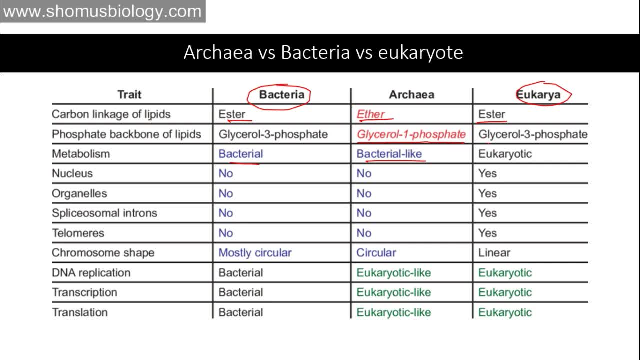 these two trait, the lipids and the lipid link with the phosphate Backbone, are similar between bacteria and eukarya. so this to have similarity, archaea has difference metabolism: bacteria in metabolism. bacteria and archaea is similar. Now think about nucleus, absent in both bacteria. 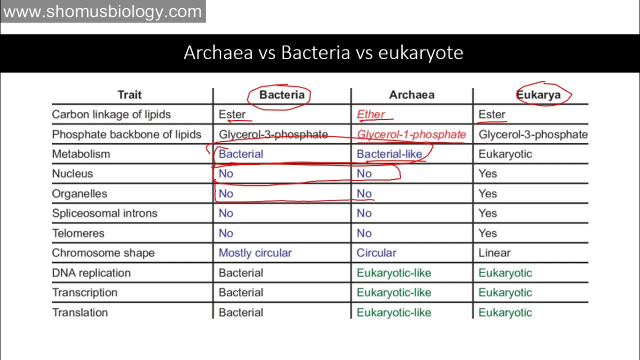 and archaea, so they have similarity: organelles not present in bacteria and archaea. They have similarity: spliceosomal introns, so there is no introns present in bacteria and archaea. They have similarity: telomeres: no telomeres found in bacteria and archaea. similarity: chromosome. 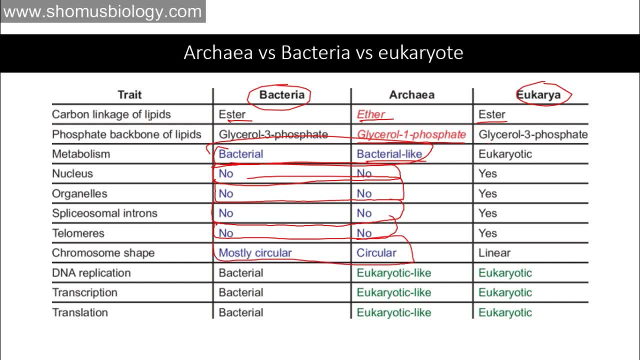 shape. bacteria and archaea are mostly circular similarity, while eukarya linear DNA replication- Now from here, DNA replication, transcription and translation- bacteria has a bacterial replication, bacterial transcription, bacterial translation process, while archaea and eukarya have similarity in replication, transcription and translation. Okay, so think about it. We have found few. 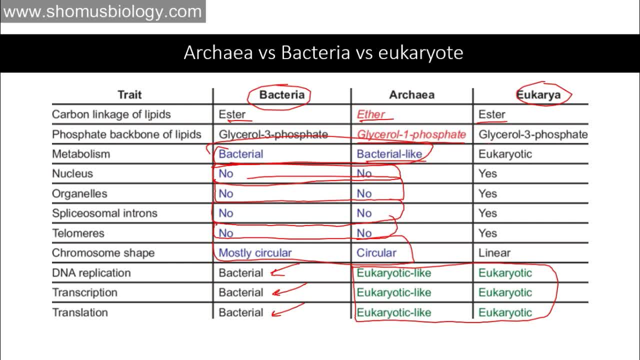 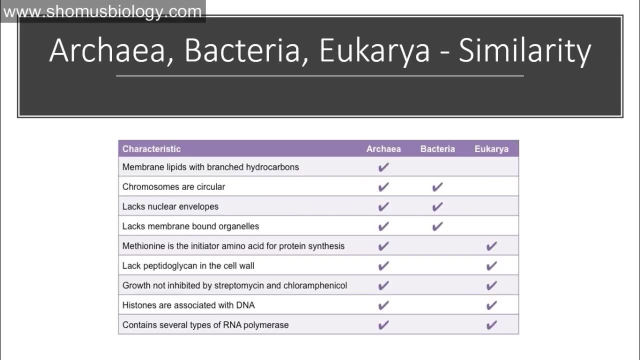 properties which are similar between bacteria and archaea. We have found few properties similar between archaea and eukarya and we have found few properties similar between eukarya and bacteria. that is only this to carbon link linkage of lipids and phosphate backbone of lipids. Okay, 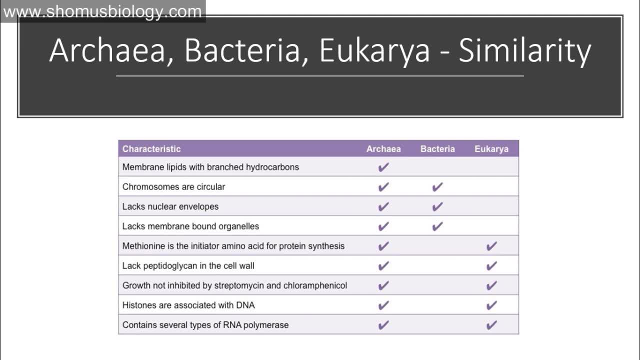 So here again the similarity is listed. Okay, so between eukarya and archaea there are more similarity, as you can see. for example, methionine is the initiator, amino acid of protein synthesis, both in archaea and eukarya. 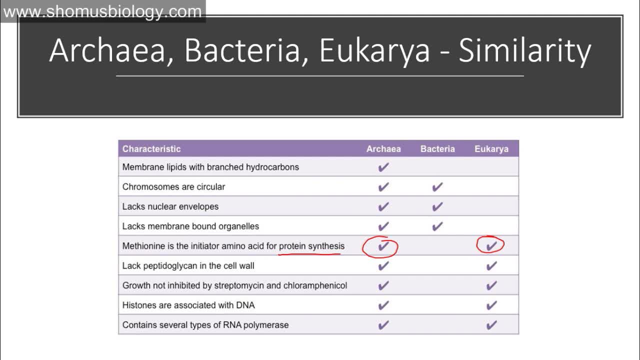 True in bacteria form a new town inude to, not through lack of pepdo glycan in cell wall in both archaea and eukarya, but bacteria has a lot of peptidoglycan in cell wall growth, not inhibited ste reduzinc chloramphen. 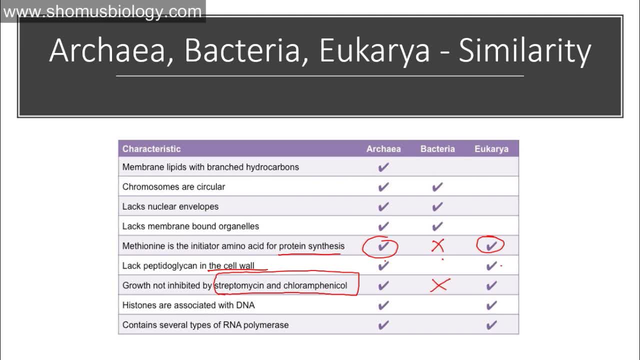 cells, the in full bacteria, but they're not going to kill and not in to稱りました dna Hi- ties, priesthood, cdV-facуса-a, ussah mouths and late C Caldwell, vallane-faloit erode. 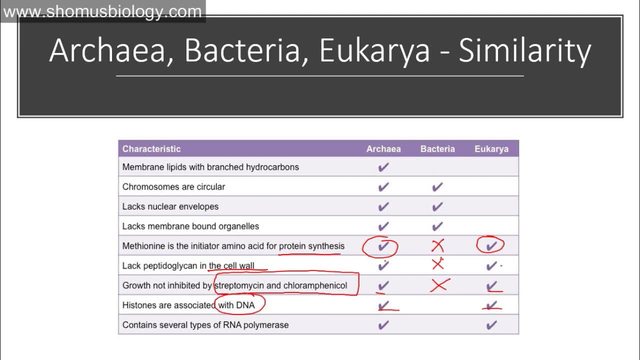 inflammasagra es ROS0114 in bacteria-not in the 1848 in cell wall. whichPPGt'sевой crawl in DNA. both in archaea as well as eukarya histones are present. histones are found. they are associated with the DNA and bacteria. they don't have any histones associated with the DNA. DNA is 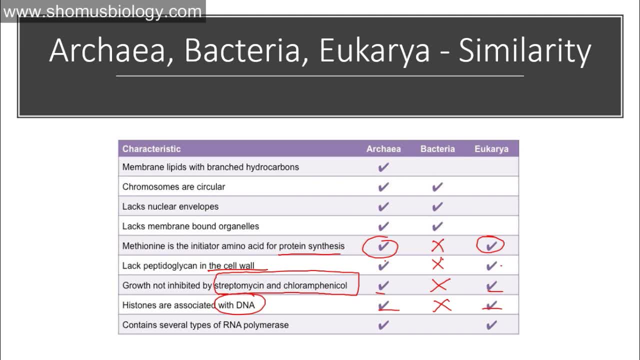 naked. inside the cytosol contains several types of RNA polymerase in archaea as well as in eukarya. they carry multiple RNA polymerase, RNA polymerase 1, 2, 3 different types. well, in bacteria there is only one type of RNA polymerase found the similarity between archaea. 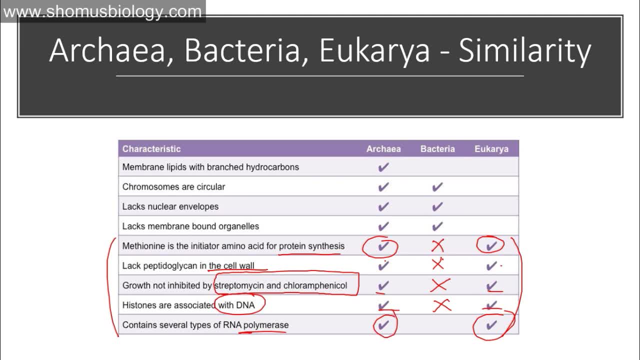 and eukaryote, but know the er between archaea and bacteria, as we know, chromosome of circular between the two nuclear, all of our absent in both membraneometals are absent in both. this is the similarity and dissimilarity between both eukaryote and archaea. if you carry a 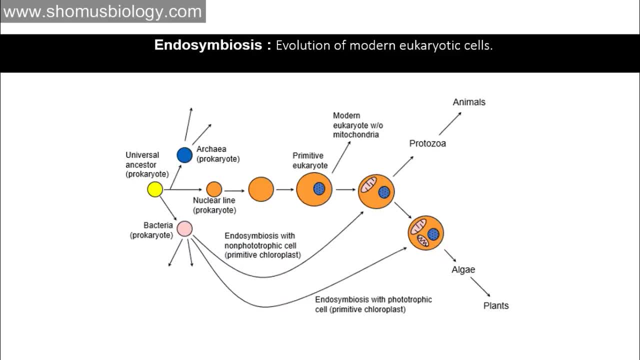 and bacteria and archaea. Now, as I said earlier that the chloroplast and mitochondria, they are nothing but prokaryotic organisms which were free living at some point of the time in evolutionary history, and then they are internalized. So this is universal, ancestral. 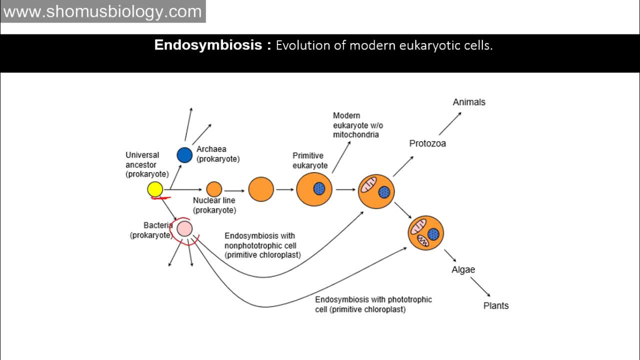 a prokaryote, from their branched into archaea, first branch into bacteria, then a second branching to archaea and eukarya. So among some of the bacteria they are this, this chloroplast or mitochondria. they are present as a prokaryotes and sooner, window eukaryotic cells are produced. 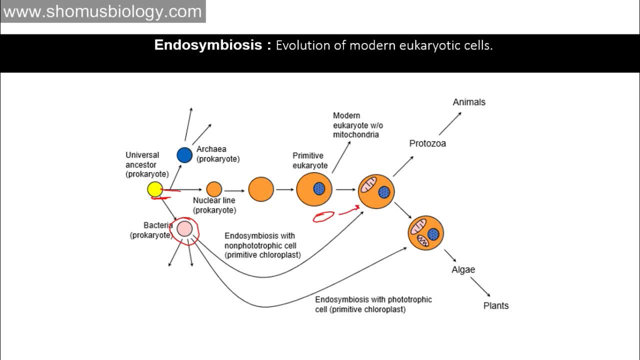 then this, this small prokaryotes, are internalized by the eukaryotic cell inside of the cell. And once they're internalized inside the cell- because you know this, this prokaryotes, they have their own genetic material and they utilize their own genetic material for the 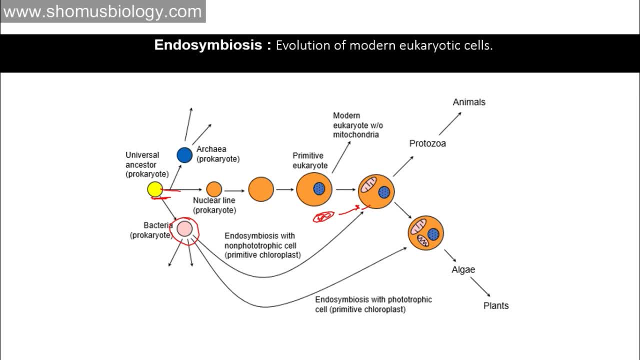 transcription and protein synthesis replication inside, So they're self replicating components. And when they start replicating itself inside the cell, inside the eukaryotic cell, so eukaryotic cell start getting benefit from these structures, for example from mitochondria. they start getting benefit of producing energy. 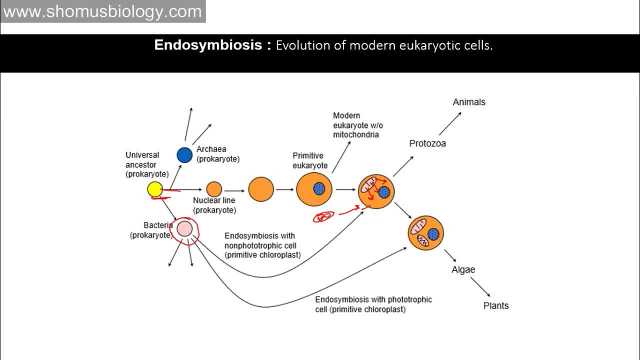 and eukaryotic cell can now get energy from the mitochondria and then can utilize the mitochondria as a powerhouse, And chloroplasts contain like this. this chloroplasts contain this chlorophyll which can be utilized by that eukaryotes. 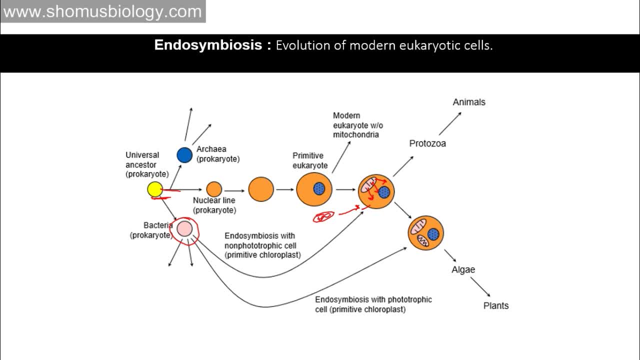 So they are going to start to to photosynthesize and produce food. So that provides them benefit. And as that provides benefit to the cell, cell utilize that and they are going to divide and replicate into two. So once the cell continues to divide into multiple cells- sooner new 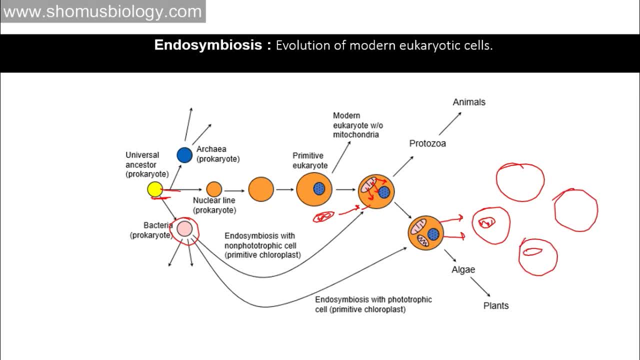 cells start containing that, that cell and mitochondria. they also get benefit mitochondria and chloroplasts. they also get benefit of receiving nutrients and other components by the cell. So it's a symbiotic relationship between this Prokaryotic cell and eukaryotic cell. that's why the prokaryotic cell remained there and 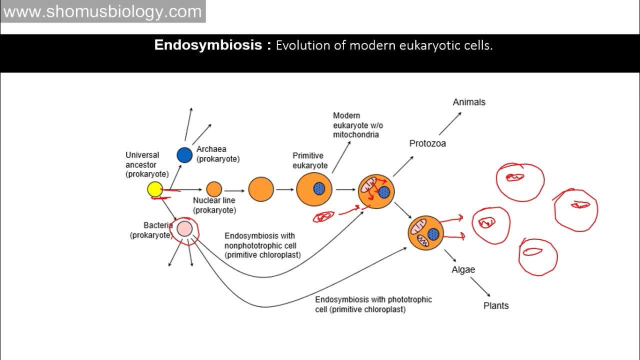 live there, So that's how we find out this. this mitochondria and chloroplasts will be a part of this eukaryotic cell. later on, And and a few of the cell which receives mitochondria became animal cells, and those received this chloroplast along with mitochondria became plant cells. 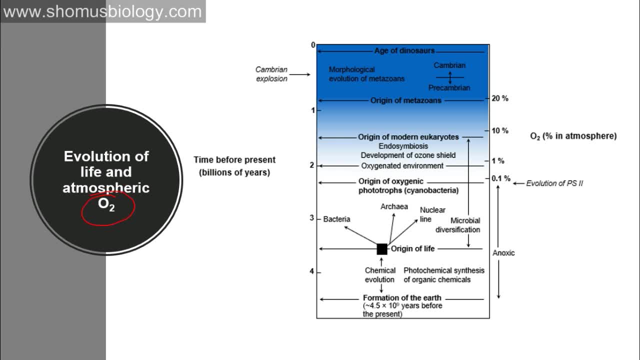 Think about the evolution of life, how oxygen, atmospheric oxygen, drive it. you can think about it, that origin of lime from there after the chemical evolution, and it produced bacteria, then produce archaea, nuclear line and from the nuclear line the eukaryotes are produced later on and the microbial diversification. 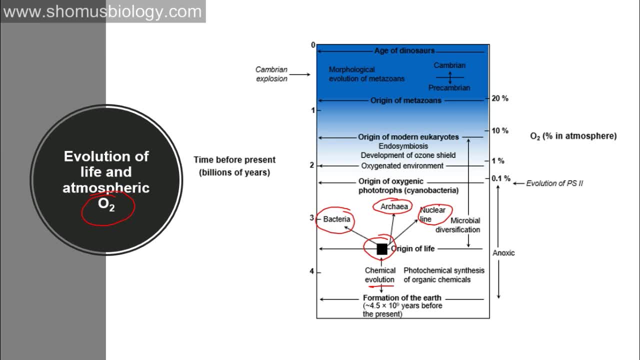 took place and, you know, small modification taken place at a time, because earlier there's a part known as anoxic environment, where the environment, the atmosphere, lacks oxygen because atmosphere filled with nitrogen, hydrogen, ammonium, this kind of gases. but now this anoxic environment is altered, it's changed and oxygen start building up and you can see the evolution of photo system to 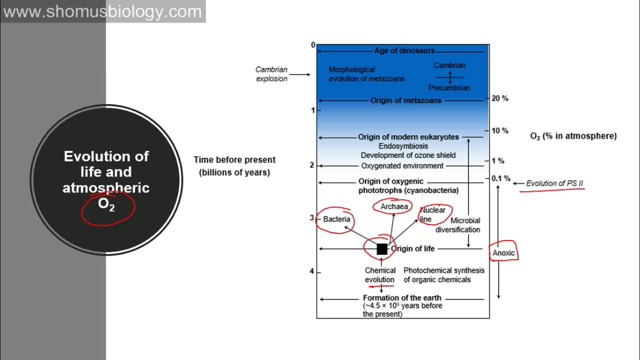 taken place and you can see that oxygen concentration increases slowly from 0.1 percent uh. the origin of oxygen in photo drops, like cyanobacteria, they start using very low amount of oxygen and then oxygen oxygenated environment where 1 percent of the oxygen then origin of. 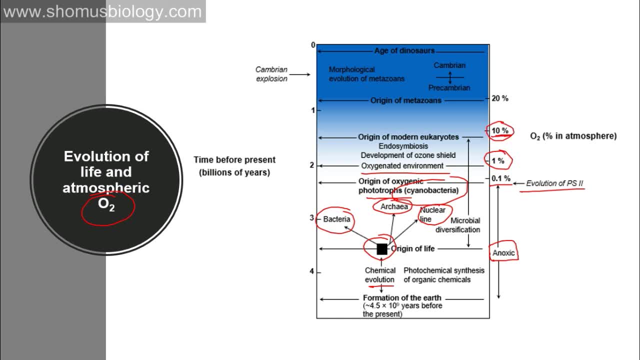 modern eukaryotes, when the oxygen concentration percent is 10 percent and now near about 20 percent of the oxygen origin of metazoans. so you know, the more the cells become, the more the origin, the complex the the body of the organism become, uh, the more oxygen demand they start to, they start. 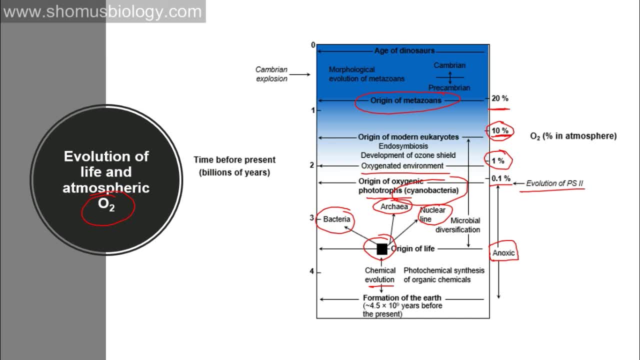 to do so. more oxygen demand means 20 percent, ultimately, at the end, 20 percent of the oxygen. 20 percent oxygen saturation in atmosphere leads to the utilization, uh like, of the oxygen, and metazoans utilize the 20 percent of the oxygen and they start growing and uh that that time is uh is a pre-cambrian to cambrian. 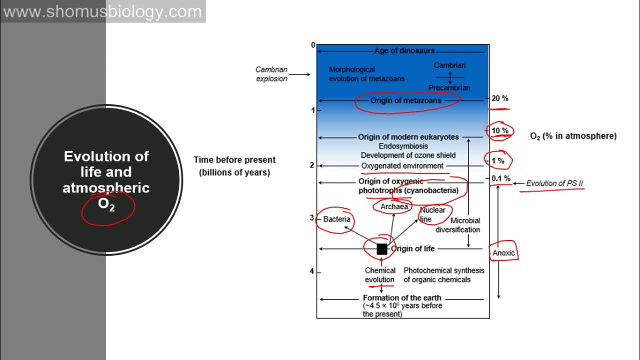 time where the morphological evolution of metazoans take place and then become the age of dinosaurs later on. okay, so these are the things that we can see in the photo, so we can see that the parasites are being survived and that the mitra is now kept in time. UV市 �pie Travel. 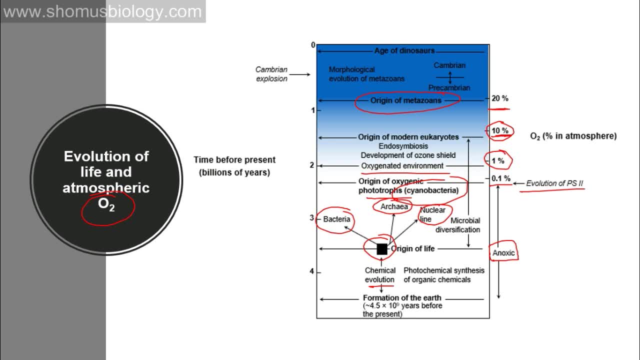 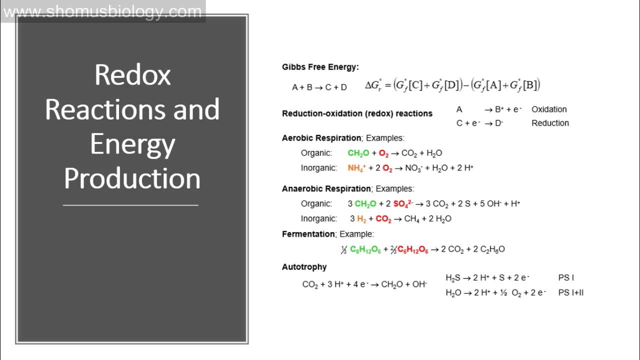 nake with 10 years before. the present time is then after chemical evolution, origin of life at the inel zit environment and slowly the in ox- a environment starting from 0.1 percent utilized by the cyanobacteria and then goes to 20 percent- were in the meta zones originated. 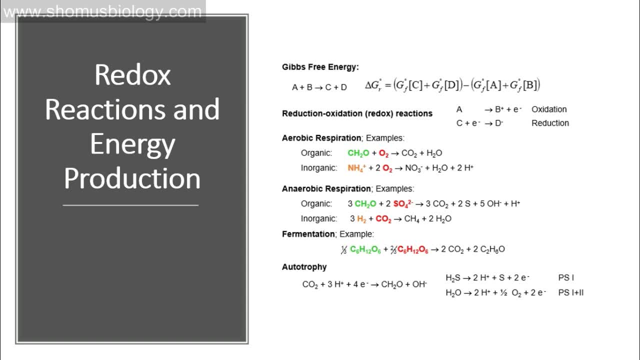 result. no, to take away's from about these microorganisms and how they are utilising energy. They are mostly utilising redox reactions for the production of the energy, And when we say redox, that means reduction and oxidation, And the easy way to remember is oil rig. Oxidation is losing. 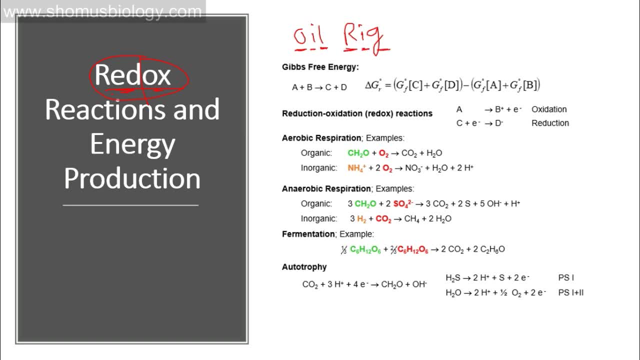 electron reduction is gaining electron. So the Gibbs free energy change is listed, which we are not concerned to talk about, but think about it. The redox reactions for an oxidation is when the component A is converted to B plus and electron is removed while in reduction. 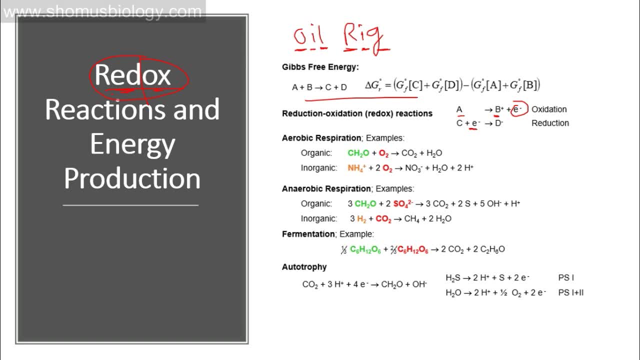 electron is taken, Electron is used. Okay, Remember that in oxidation electron is produced. in reduction electron is utilised. So aerobic respiration. example: organic and inorganic. organic: When the CH2O oxidizes, the electron is removed. When the CO2O oxidizes, the electron, 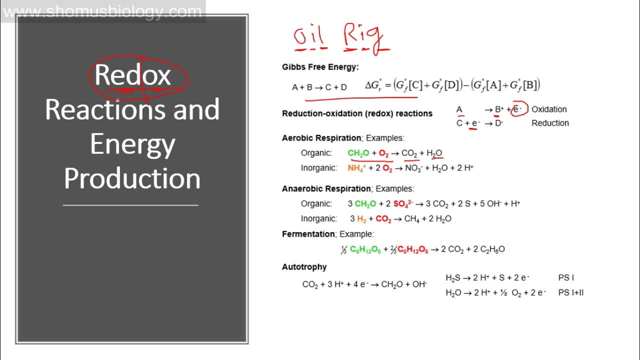 is removed, Oxygen is utilised to produce carbon dioxide and water Inorganic, when ammonium and oxygen is utilised to produce nitrate water and hydrogen. Okay, So both are oxidation reactions for aerobic respiration. For anaerobic respiration, we can use the organic compound. 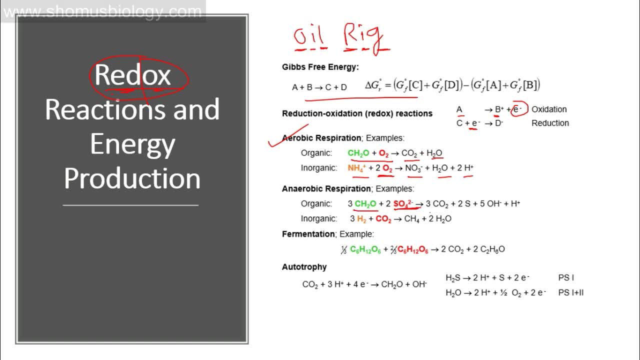 hydrocarbons Sulphate is used to produce carbon dioxide, sulphur, hydroxyl and hydrogen that can be reduced like converted to water later. This is the organic method And the second method. if you use inorganic gas like CO2 and hydrogen, together produce methane. 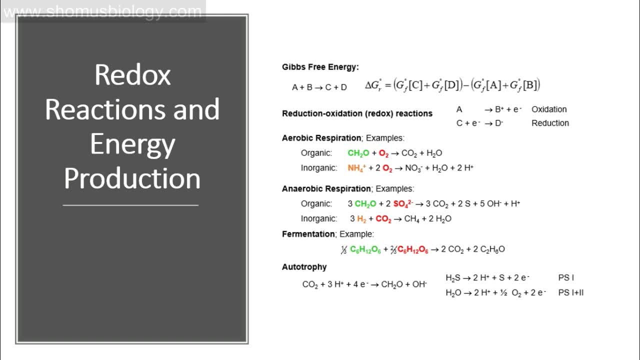 and water. On the other hand, if you think about the fermentation, fermentation take place in anaerobic condition only. So in anaerobic condition we've seen two examples where we use organic material and when microbes can use inorganic material, but in fermentation. 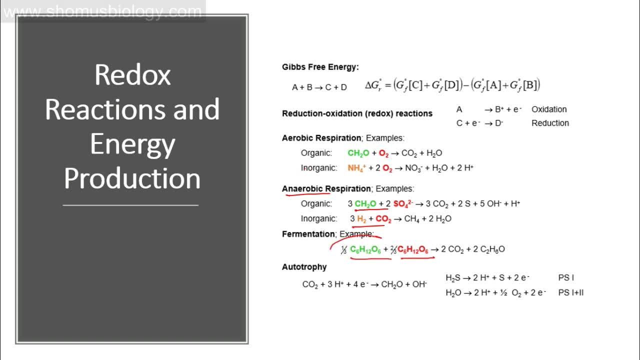 also, they utilise sugar. You can see C6H12O6, the sugar components, and they can also produce carbon dioxide, And the hydrogen is also used to produce carbon dioxide. So inorganic gas like CO2O and hydrogen produce methane and water. On the other hand, if you think about the fermentation- fermentation- 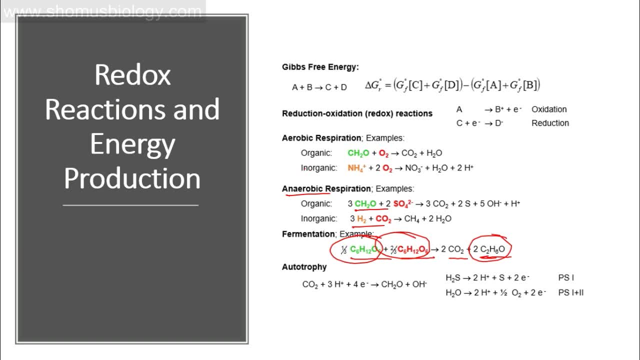 the hydrocarbon chain, In this case you know aldehyde, and from there it can produce ethanol as a fermented product or lactic acid as a fermented product. So these are all regarding microorganisms were utilising inorganic or organic in carbon source. But apart from that, 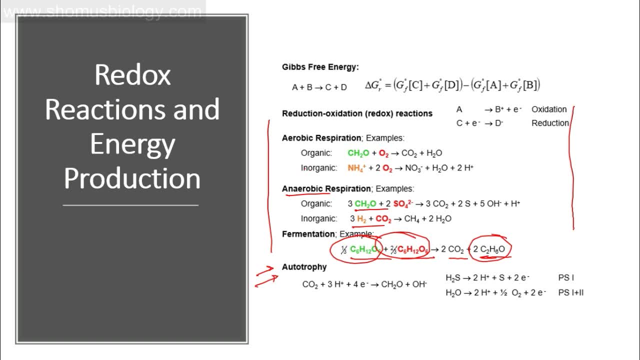 there are situations known as autotrophy. Autotrophy: a situation where carbon dioxide is used and the energy from sun- energy from sun- is used. Okay, and there are photosynthesis systems that help microorganisms to harvest the sun energy. So there are two photo system. 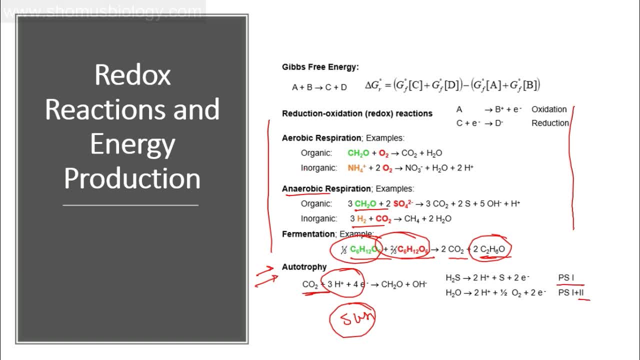 photo system one and photo system. to few microorganisms have only photo system one. few of them have photo system one and two together. Now, either way, this photo systems are filled with a photo pigments known as, like chlorophyll, photo pigment or chlorophylls, So the chlorophyll is also. 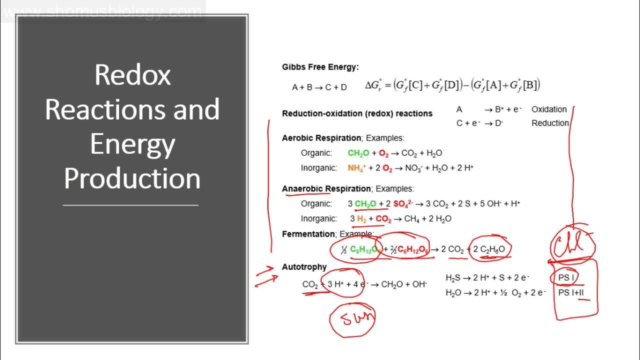 known as photo pigment or antenna pigment, receives sunlight and gets excited. when it get excited, then they are going to release electron and electron gets transferred from one photo system to the other in the higher energy state and there are electron carriers embedded into the membrane of chloroplast- I mean not the chloroplast membrane membrane. 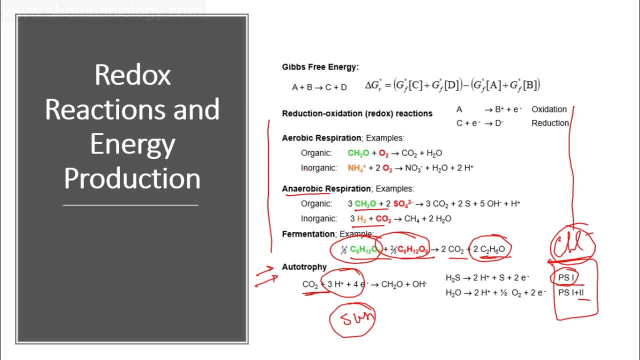 of the thylakoid and as a result of which that leads to a process in production of energy That produces ATP, which is a energy currency inside the cell, which is which can be utilized by the cell quite easily. So ATP can be utilized. So this is a photo reaction or light reaction.